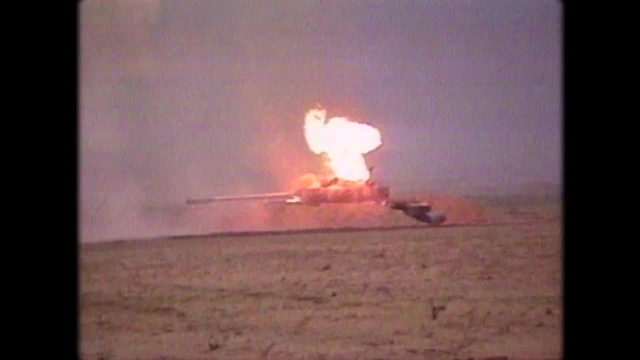 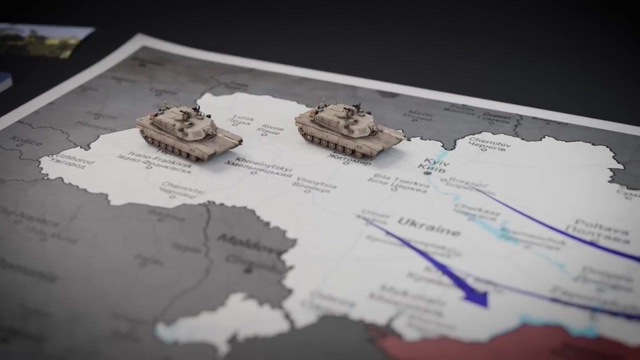 It easily dispatched the lower tech Soviet supplied tanks of the Iraqi army. Sometime this year it's expected that the US will deliver a battalion of 31 M1 Abrams tanks to Ukraine to once again face off against the Soviet tanks it was designed to battle. 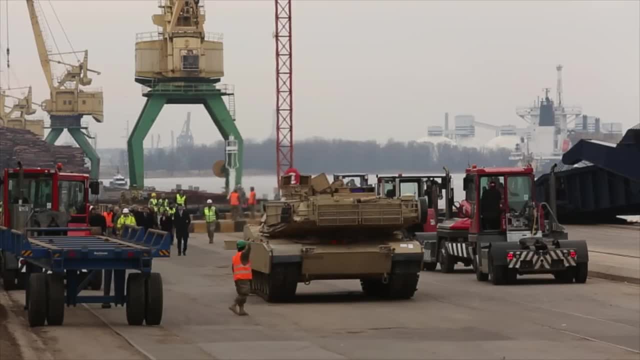 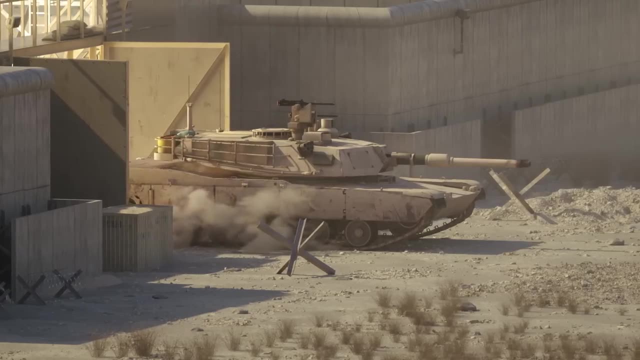 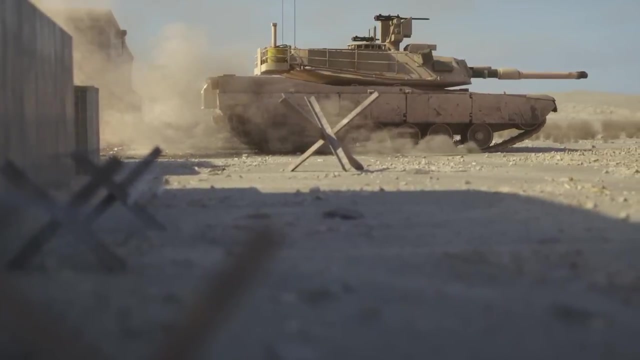 Ukrainian army will need training to maintain and operate these new tanks, because they are like no other tank And although this tank is over 40 years old, it's still more than capable of holding its own on the battlefield, thanks to continual modernisation and forward thinking design. This is the insane engineering of the M1 Abrams. 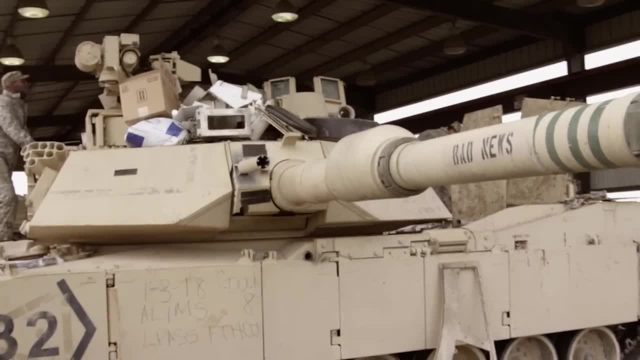 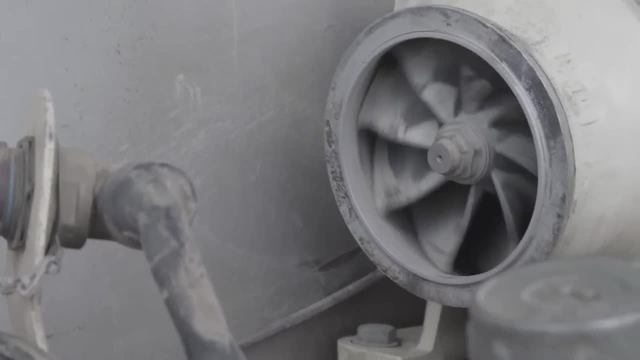 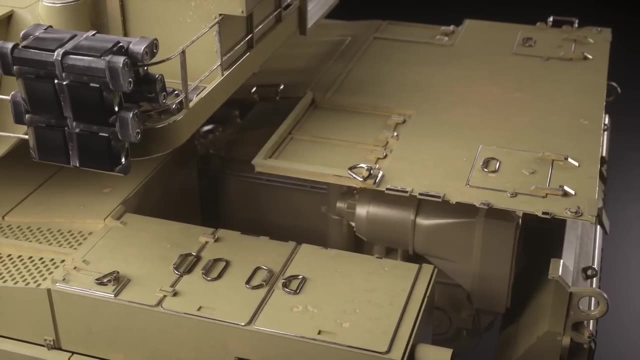 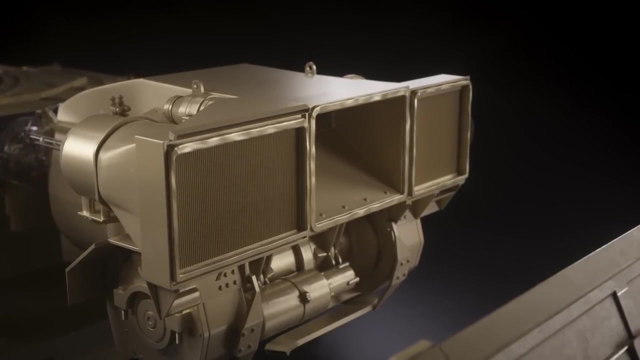 M1 Abrams, M2, M1 Abrams, M2, M1 Abrams, M1 Abrams. upon engine startup sounds more like a military aircraft getting ready to take off A terrifying increasing pitch. as the engine revs up to speed, The whirring sound emanating from the rotating turbine blades hidden inside. 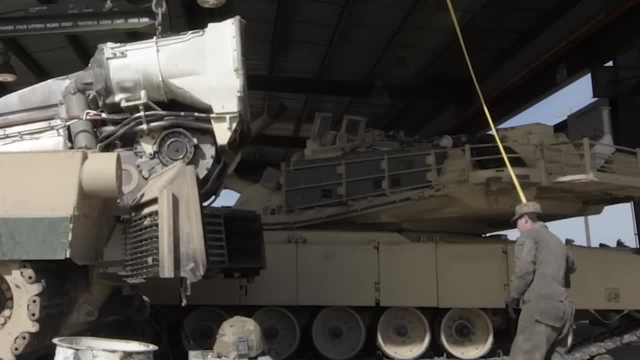 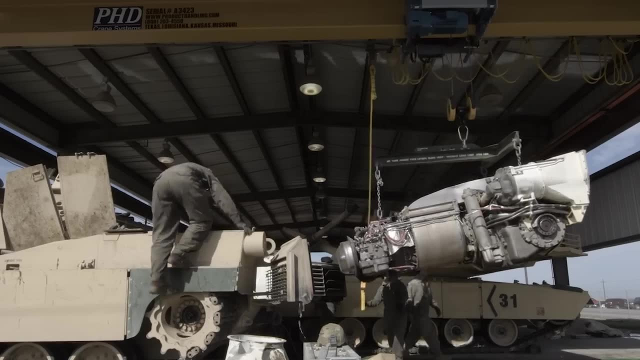 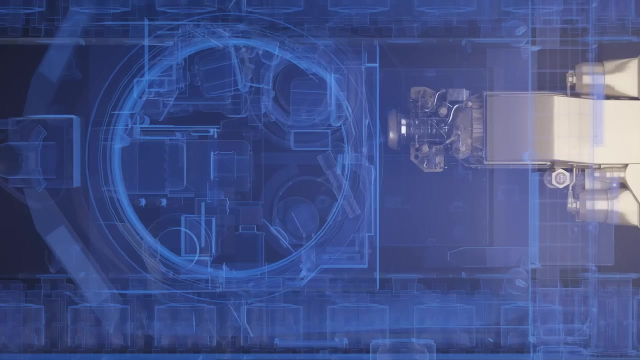 The turbine engine, typically used for jet aircraft, is an engine designed for high speed operation with minimal weight- A counter intuitive choice for a heavy battle tank. So why was it chosen? The turbine engine would give the M1 two huge advantages: They are much lighter than an equivalent diesel engine, weighing just 1.1 tonnes, and developing. 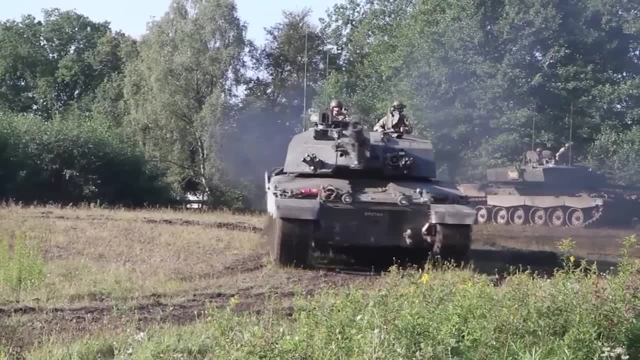 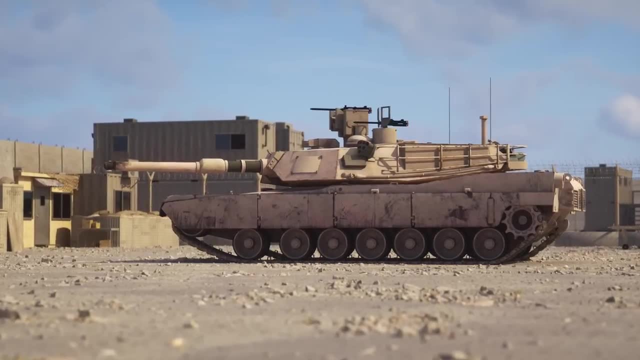 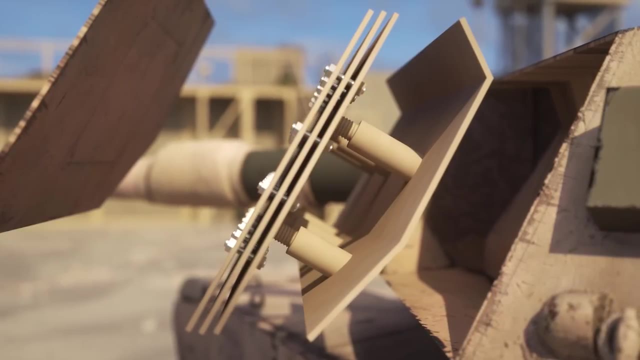 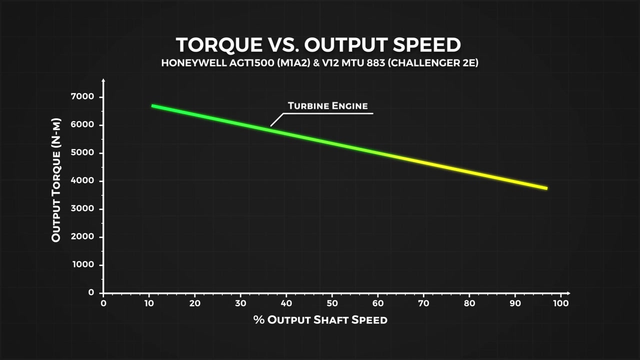 1500 brake horsepower, The V12 diesel engine of the Challenger 2 produces 1,000 horsepower. This compactness and extreme high power to weight ratio allows the M1 to stack on layers of armour without sacrificing acceleration or top speed. We can plot torque vs shaft speed of the Honeywell AGT-1500 turbine engine of the M1 against. 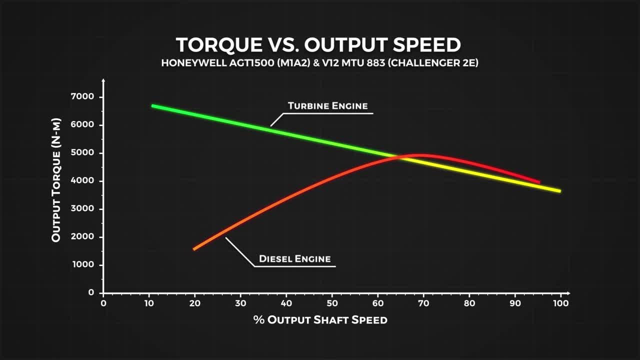 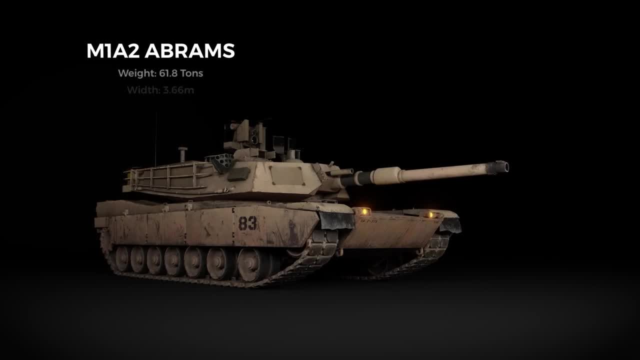 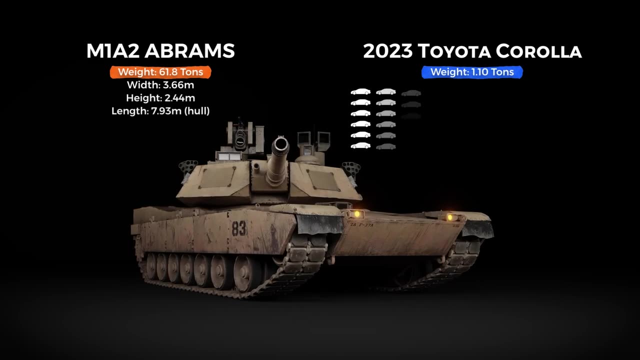 the V12 MTU-883 of the Challenger 2E and we can see the turbine has a massive torque advantage at lower shaft speeds. In its lightest configuration, the M1 weighs 61.8 tonnes. A typical Toyota Corolla weighs 1.1 tonnes. that's equivalent to 56 Toyota Corollas. 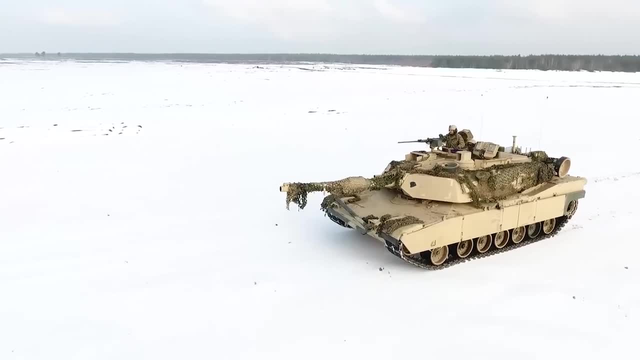 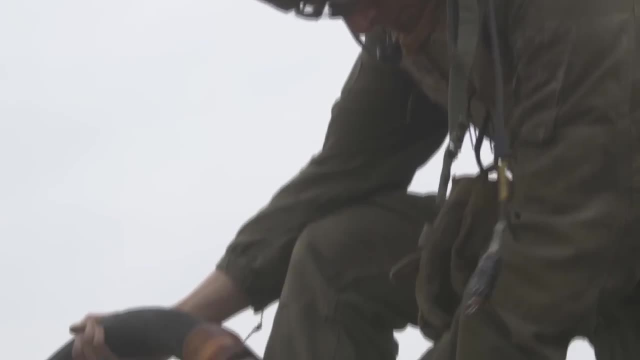 Yet this thing can accelerate from 0 to 32 kilometres per hour in just 7 seconds, with a top speed of 72 kilometres per hour. The M1 Abrams primarily uses diesel fuel, as diesel can act as an additional layer of armour. 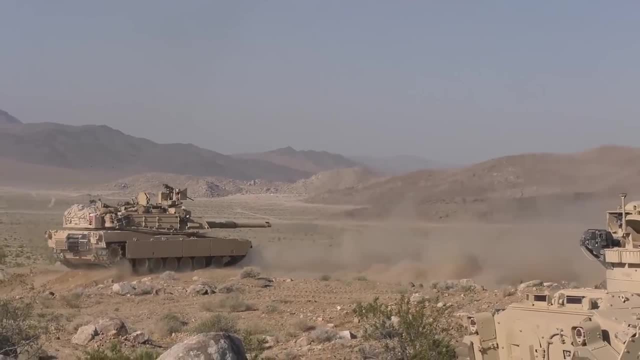 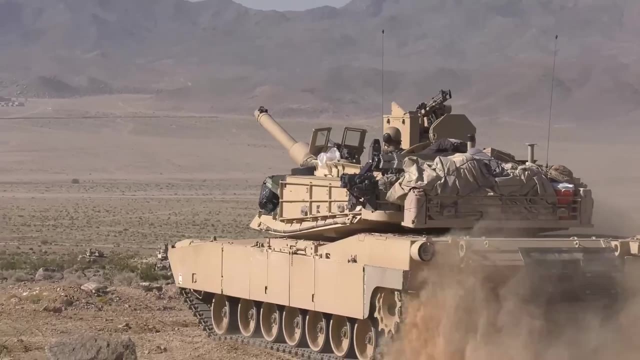 Fluids are extremely good at absorbing energy from explosions and kinetic energy weapons. They are most effective against shaped charges, and tanks carry a lot of liquid in the form of fuel. It may seem counter-intuitive to use fuel as protection from an explosion, but diesel 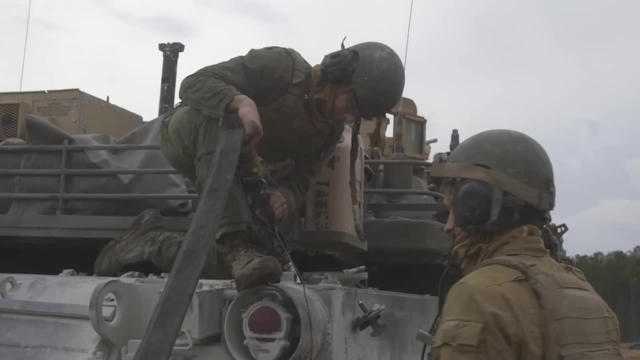 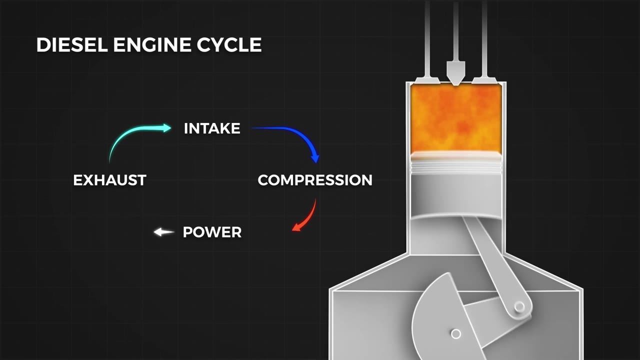 fuel is not very flammable. In fact, if you throw a lit match into a puddle of diesel, it will put the match out. Diesel engines require immense pressure and a sustained flame to ignite. because of this, diesel can be used with relative safety as armour. 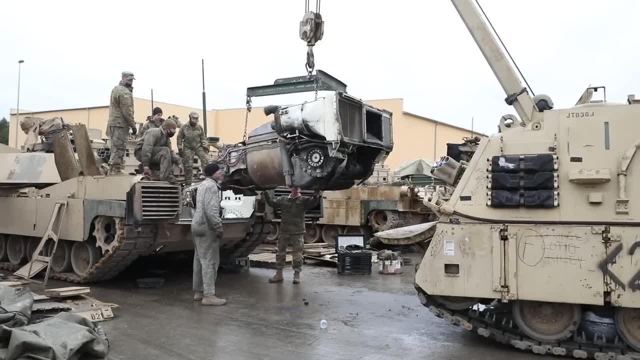 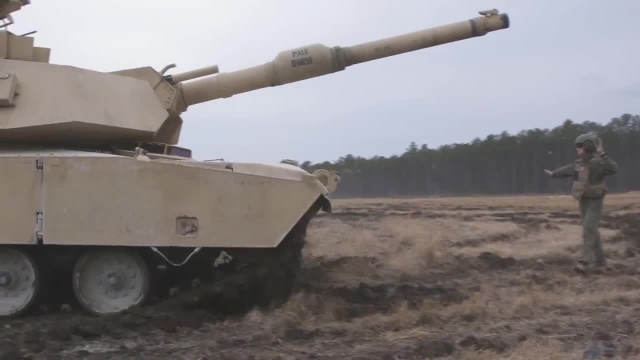 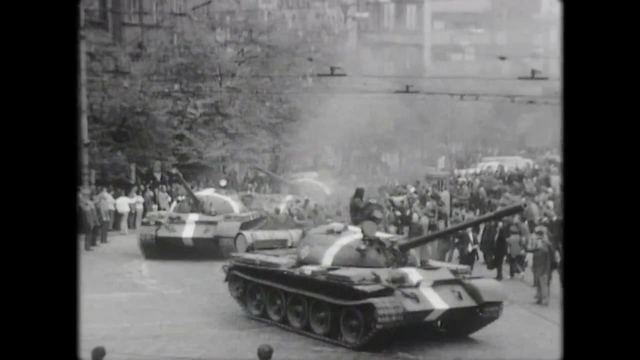 However, the turbine engine can also operate on most fuel types. This is a huge advantage in military logistics, making joint operations with NATO vastly easier. In the years following World War 2, the Soviets favoured diesel compression ignition engines. The Western Allies used a mixture of both gasoline spark ignition and diesel compression. 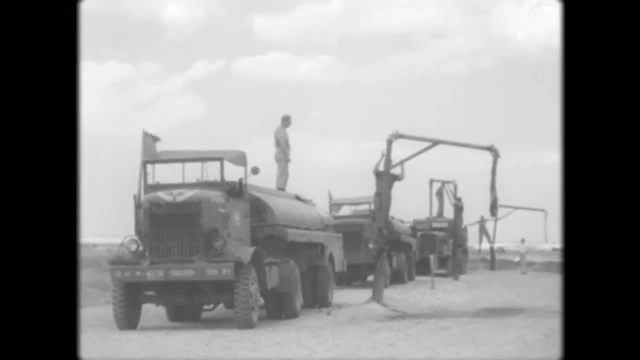 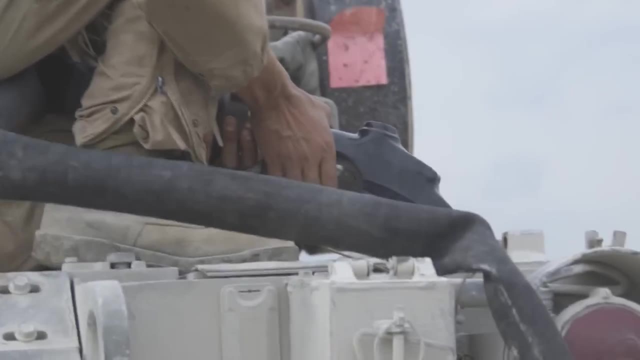 ignition. Transporting fuel is one of the latest technologies in the world. In the early 1980s, diesel engines were used to transport fuel. In the early 1980s, diesel engines were used to transport fuel. The M1 can run on marine diesel, gasoline or even kerosene if needed, which not only 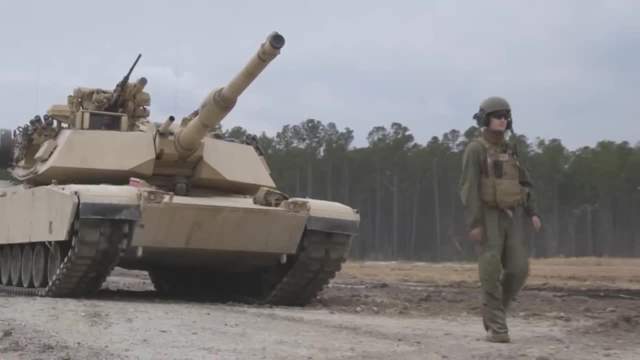 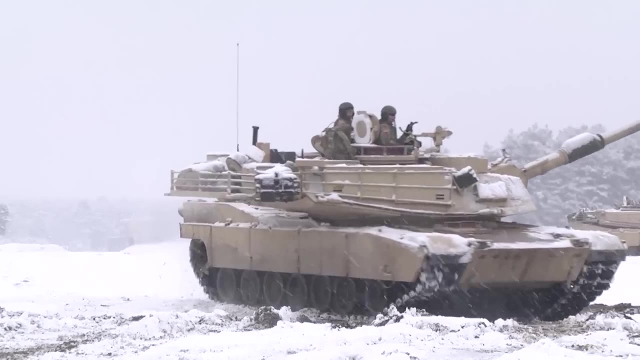 makes it easier to procure fuel in a war zone, but comes with the added bonus of helping the M1 operate in hot or cold weather, dealing with the wild swings in temperature that Ukraine can expect throughout the year with ease, Where diesel fuels can crystallize at low temperatures. 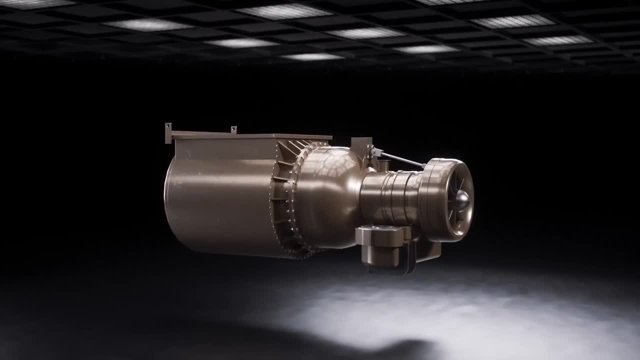 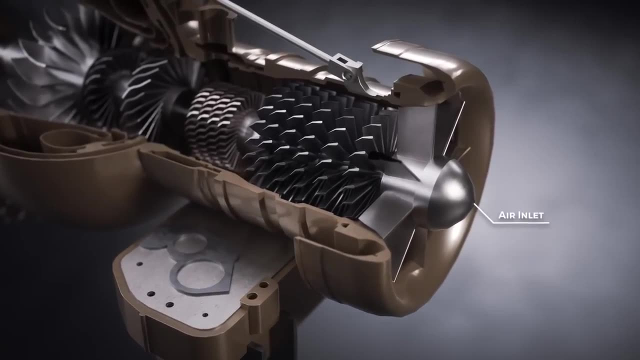 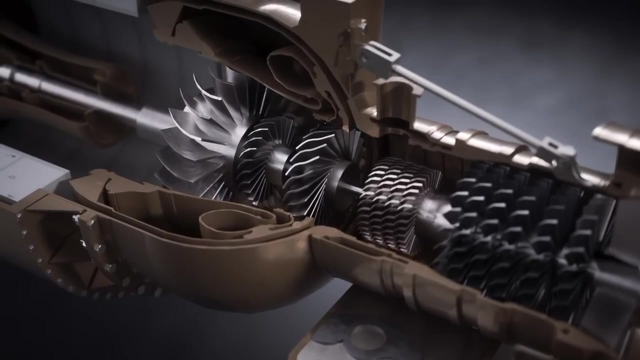 seen, can be used instead. The turbine engine of the M1 works similarly to aircraft engines, with some important differences. Air enters the engine here, where it is compressed by the low pressure compressor and then the high pressure compressor, each individually driven by separate turbine stages. 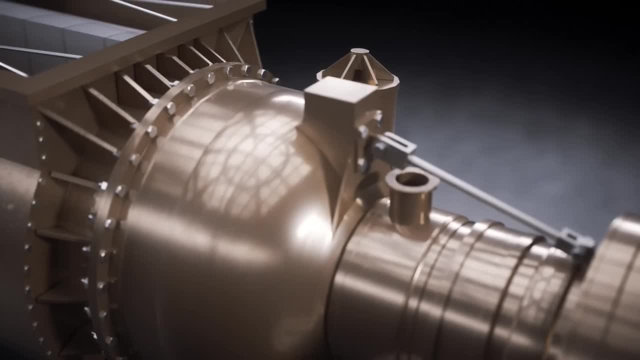 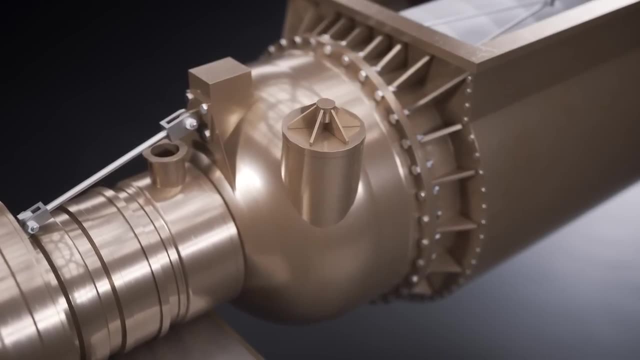 These turbine stages are driven by the combustor, which works a little differently to typical aircraft combustors. It is mounted perpendicularly to the engine and protrudes out of the engine. This makes maintenance access to the combustor easier, with only a simple bolted cover needed. 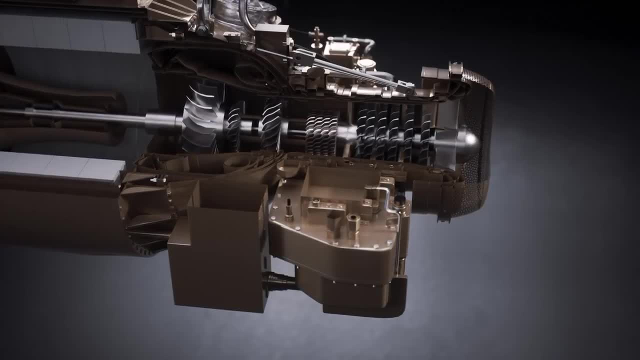 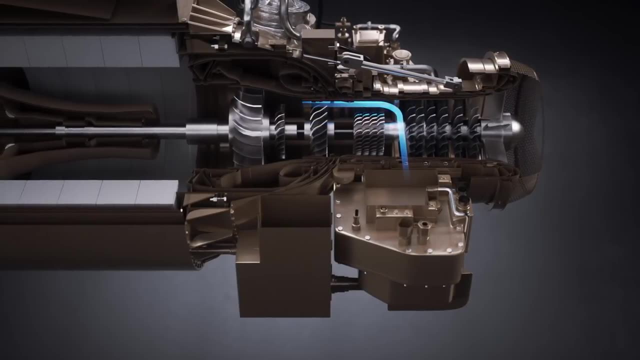 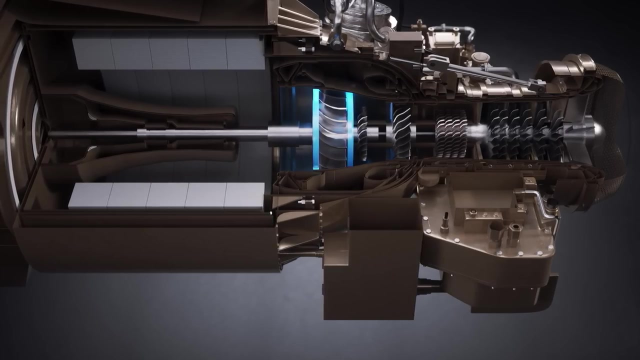 to be removed. There are two driveshafts in this engine: A secondary driveshaft, driven by the high pressure turbine, which runs forward to an accessory gearbox that runs things like compressors, electronics and hydraulics. The main driveshaft, driven by a dedicated power turbine, which is not connected to the 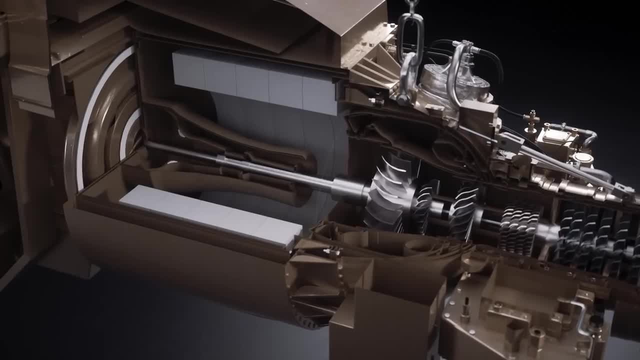 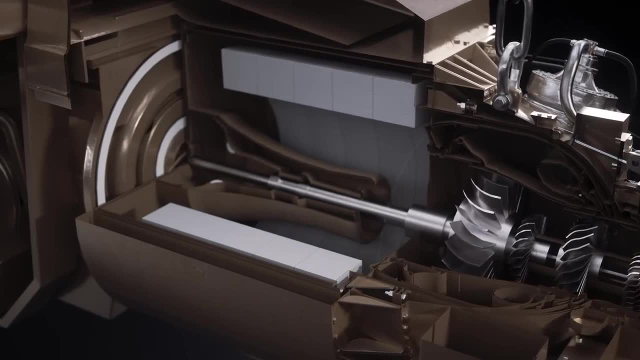 compressors, It runs rearward to the tank's drive sprockets. This primary driveshaft and it's reduction gearbox is surrounded by something called a recuperator. This is the biggest difference between this turbine engine and a typical aircraft jet engine. 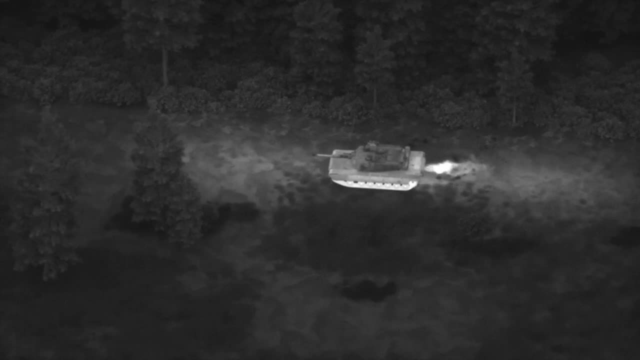 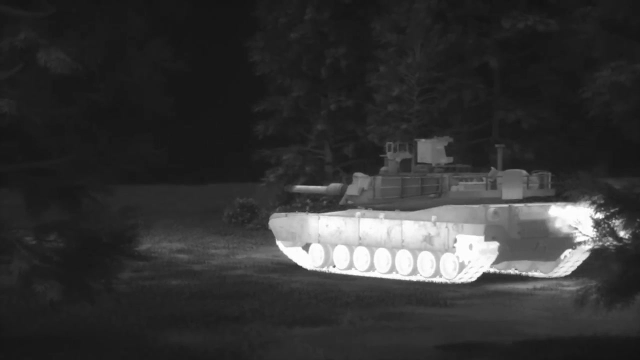 We don't want the hot exhaust of this engine spewing out like a jet engine. The heat signature this would create would be a giant beacon for heat guided missiles and give the tank's location away to any enemy using thermal vision. We also don't want to waste the heat. 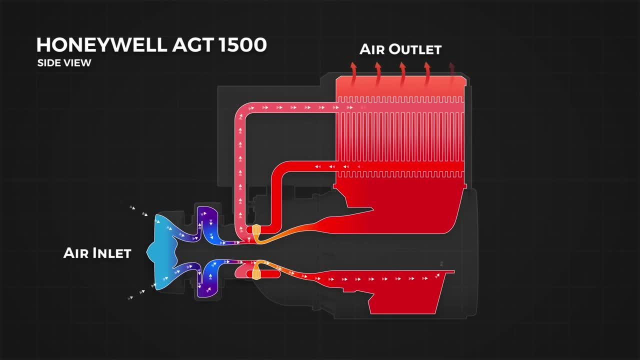 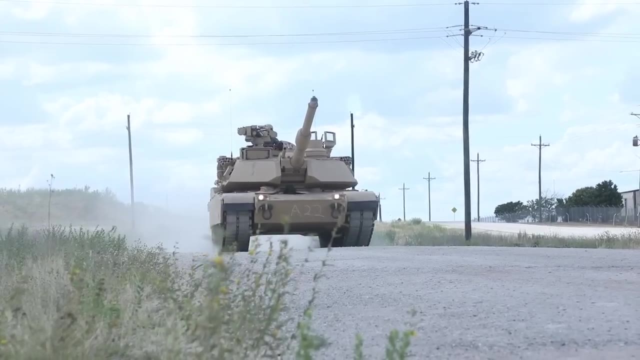 The recuperator is essentially a giant heat exchanger. Air coming from the compressor stage is passed through it, where it is heated by the exhaust before entering the combustion chamber. This lowers the heat signature of the exhaust and increases fuel efficiency, Transferring more heat energy back into the engine instead of losing it to the atmosphere. 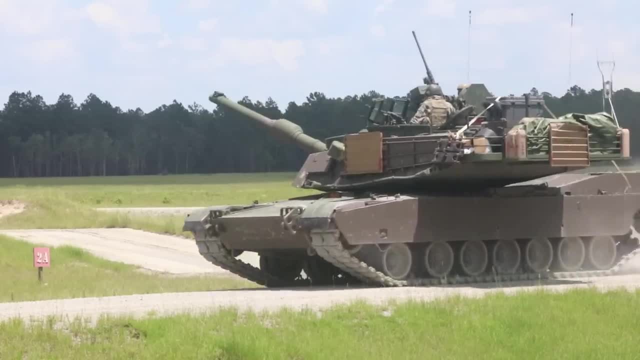 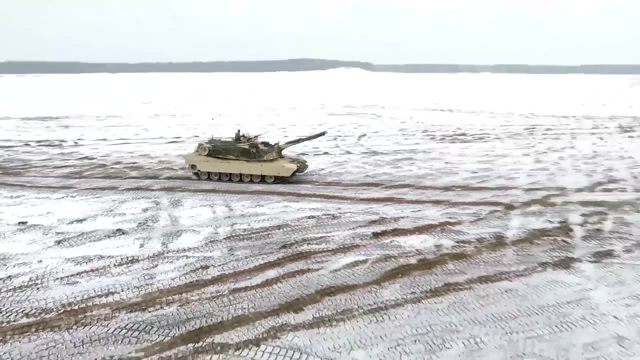 But the M1 Abrams is still a thirsty machine, even by tank standards. The turbine engine uses twice the fuel. The fuel is a comparable diesel engine per kilometre, Where the M1A1 consumes around 4.2 litres per kilometre while cruising at 40 kilometres. 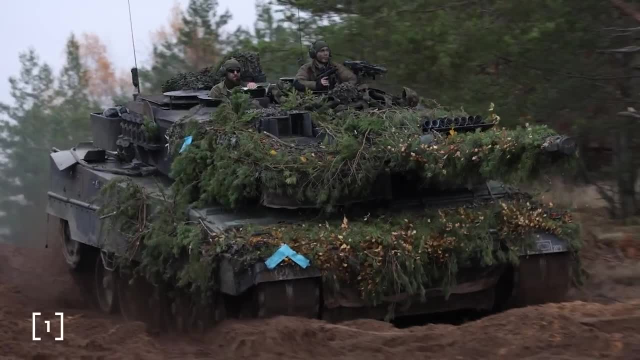 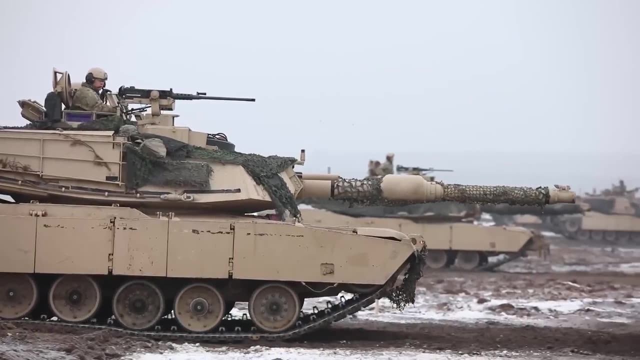 per hour. the Leopard 2 consumes 2.2 litres per kilometre, But the US military deemed this issue a cost worth paying for the capabilities the turbine engine provided, Allowing the M1 to carry an obscene amount of armour while keeping its acceleration. 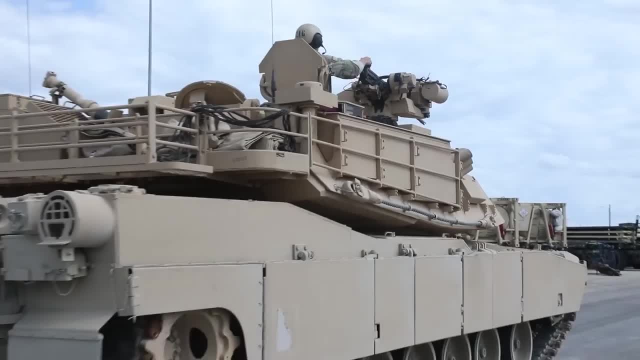 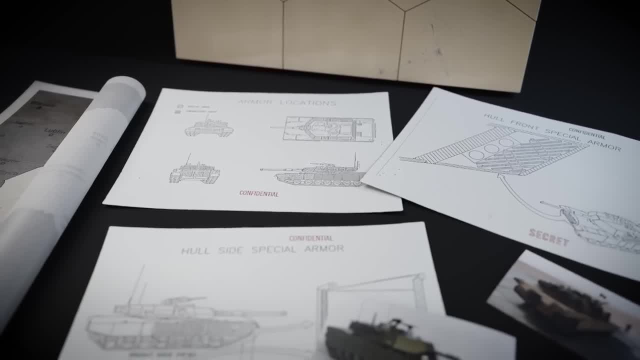 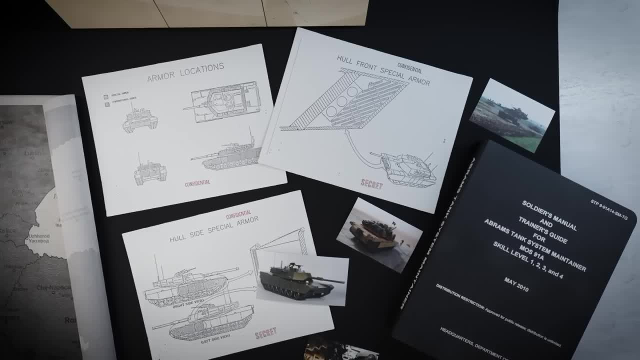 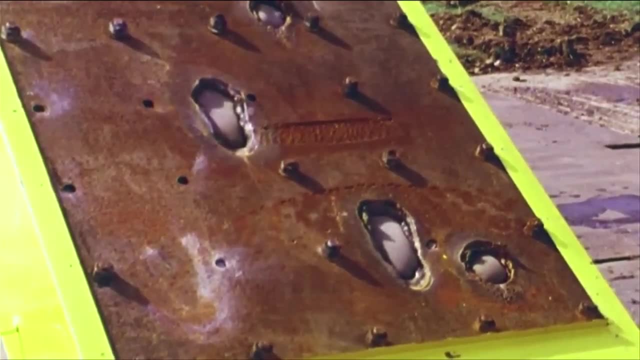 reasons, but there is a great deal known about the science and nature of its armour. It is well publicised that early M1 variants used a type of composite ceramic armour called chopum, which derives much of its ballistic resistance from an extremely hard and light 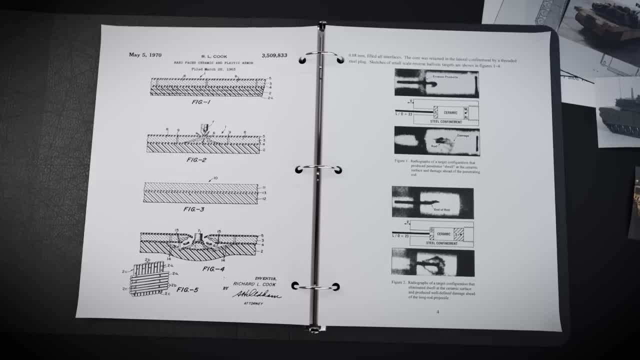 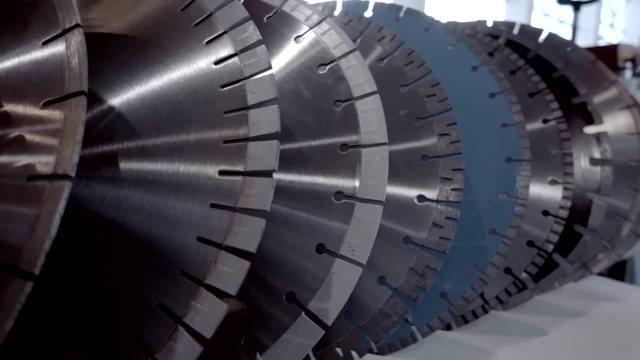 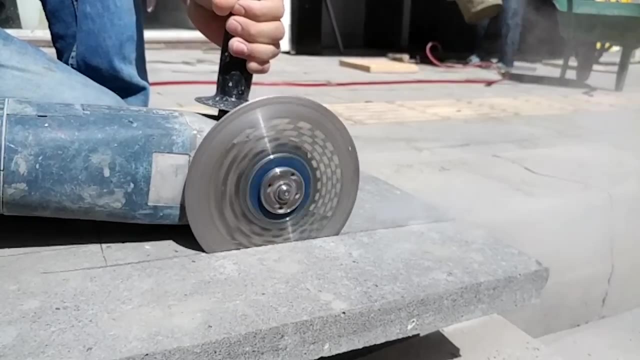 ceramic layer. Hardness in materials science is a measure of a materials ability to establish the changes, ability to resist localised deformation like a scratch. Diamonds are extremely hard and because of this industrial diamonds are coated onto cutting tools to help them cut through materials without being eroded themselves. 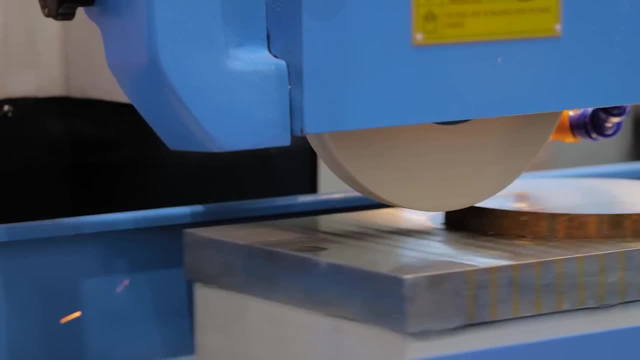 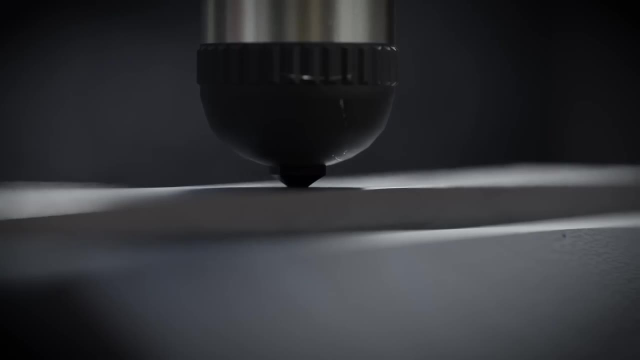 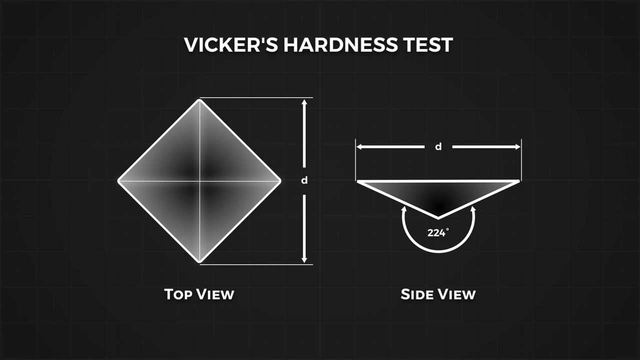 A hard material can scratch and erode a softer material. Hardness can be measured with a Vickers hardness test, which pushes a pyramid shaped diamond into the material. The hardness is then calculated by dividing the force applied by the resulting surface area of the indentation. 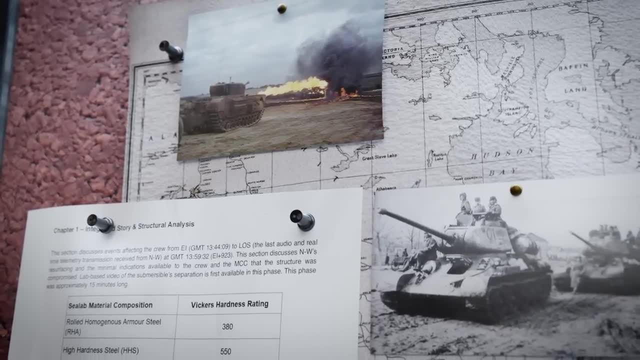 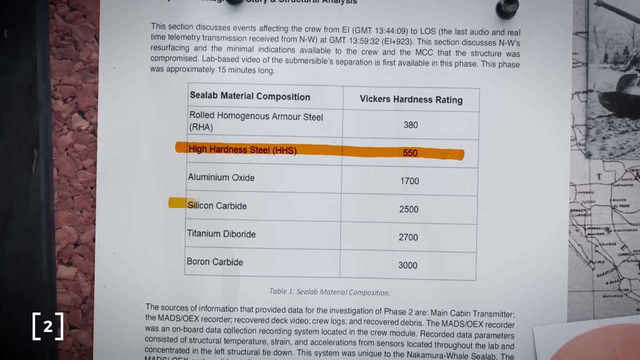 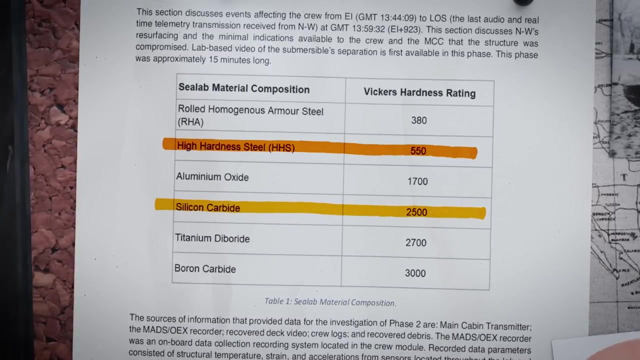 The rolled homogenous armour steel of World War 2 has a Vickers hardness test of 380.. A high carbon steel is about 550,, while a ceramic like silicon carbide offers a hardness 5 times greater, up to 2500,, while being much lighter than steel. 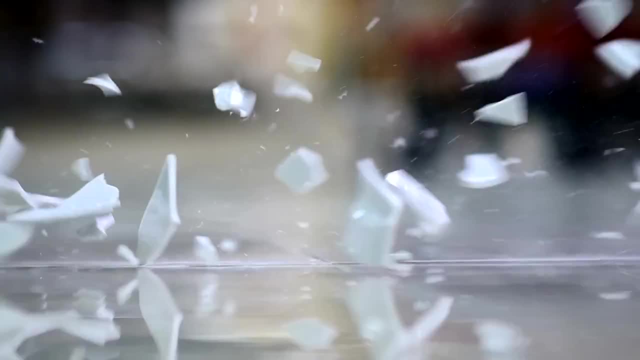 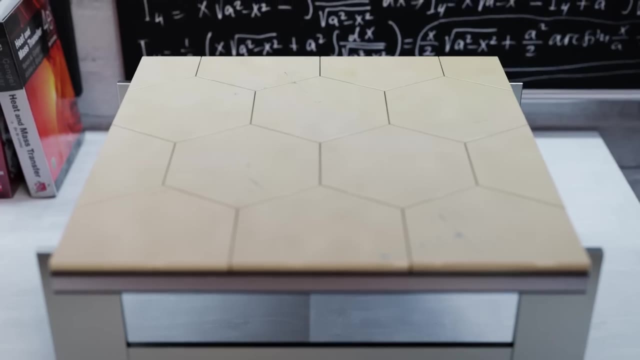 Making it an excellent candidate for armour. but anyone that has dropped a dinner plate knows that ceramics are extremely brittle. They shatter into a million pieces With little force. But this can be used to the tanks advantage when combined with a tougher metal backing. 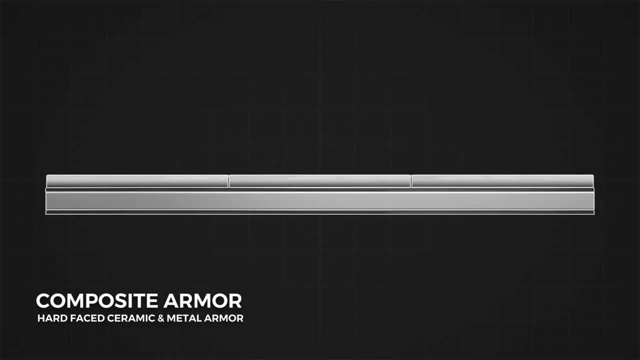 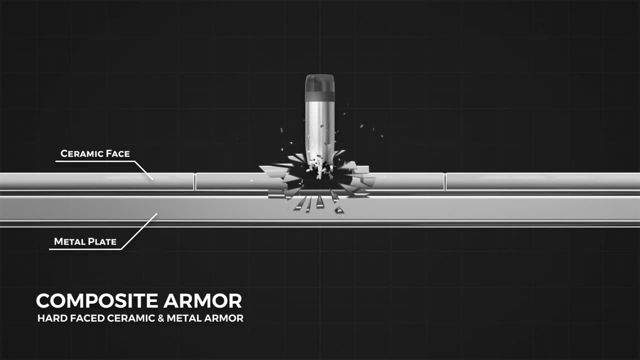 plate. In this configuration, the ceramic is placed on the outside of the metal plating, acting like an extremely hard outer shell. When a round strikes the armour, the compressive strength and hardness of the ceramic coating causes the round to fracture and break apart. 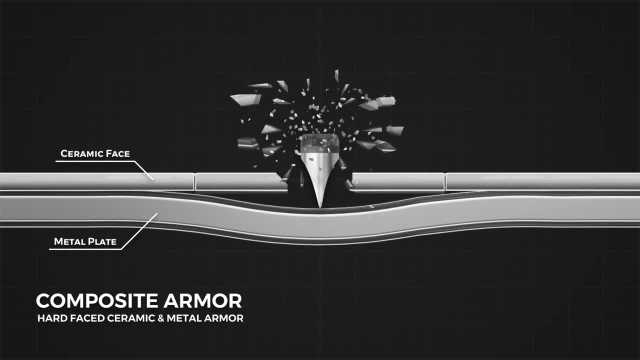 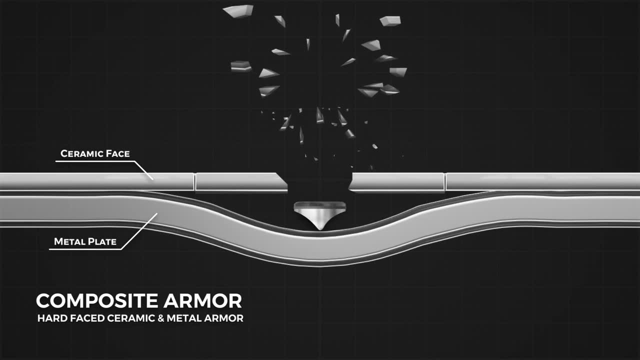 At the same time, the ceramic coating begins to fracture and fragment, spreading the energy of impact across a larger area, Which is then absorbed by the metal. Why the tougher metal plate backing the ceramic Tough? in material science means it can absorb a lot of energy without fracturing. the opposite. 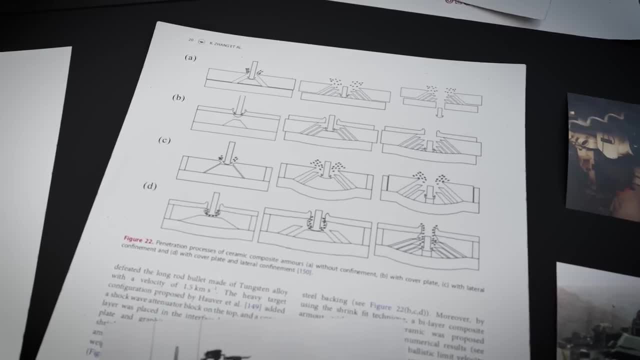 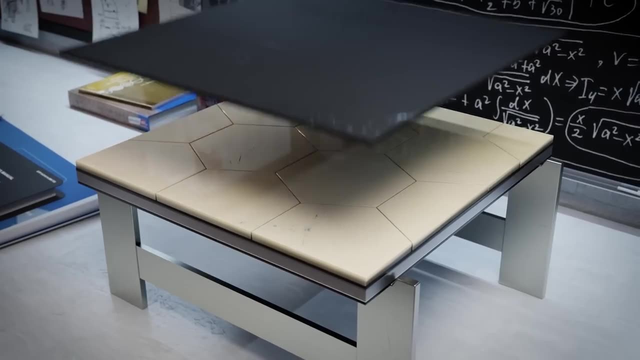 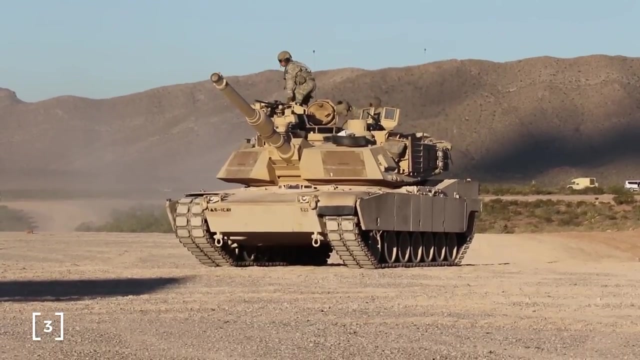 of brittle. Further research and experimentation found ceramic armour performed even better when placed under compression. This can be achieved by simply adding a face plate and bolting the two pieces together. This changes the dynamics of an impact significantly and helps immensely with resisting attack from. 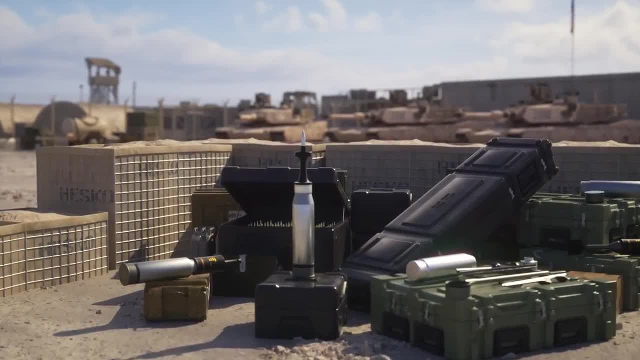 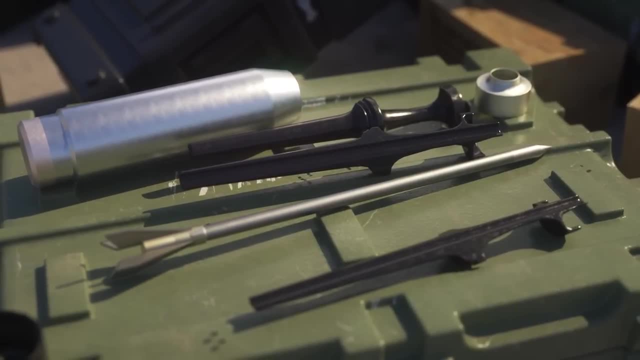 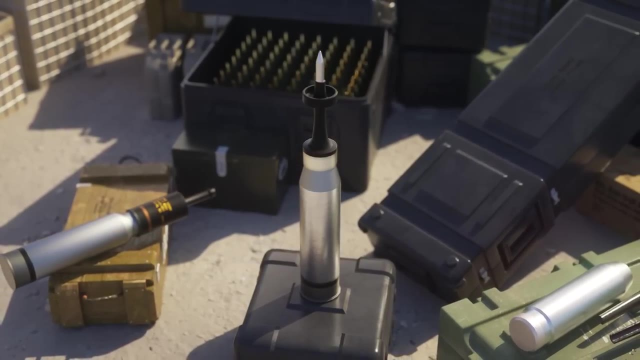 long rod kinetic energy projectiles. These are rounds specifically designed as anti-armour weapons. They are thin, long, dart, like projectiles that require a sabot to launch out of tank barrels. They are typically manufactured from high density materials like tungsten, with a thin aerodynamic shape and high density. 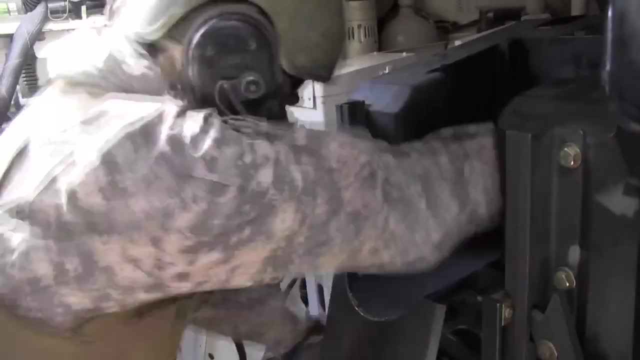 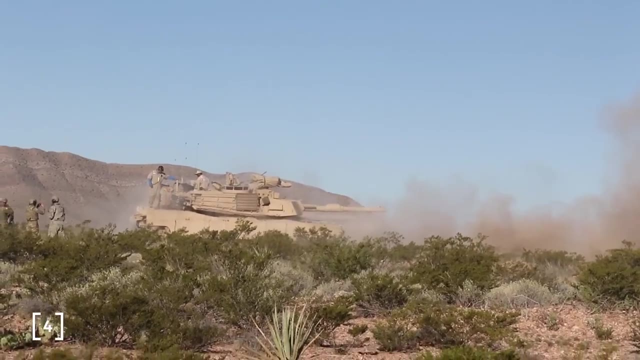 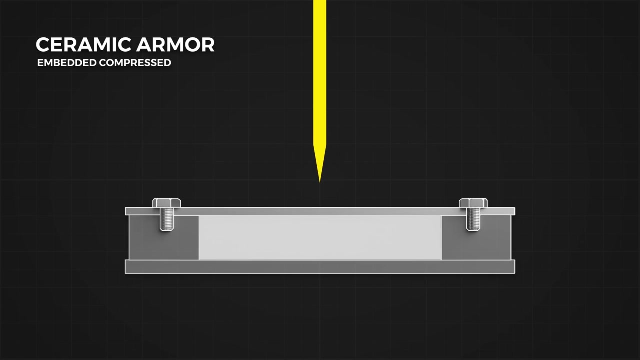 These weapons have an extremely high ballistic coefficient, allowing them to ram into targets at a distance at high velocities. They can obliterate rows of concrete walls with ease, Embedded compressed ceramic armour. Ceramic armour can defeat these kinetic energy weapons. When the long rod projectile strikes the face plate, it sends a pressure wave through the 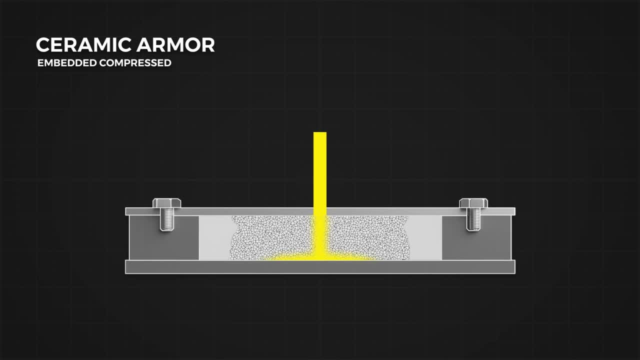 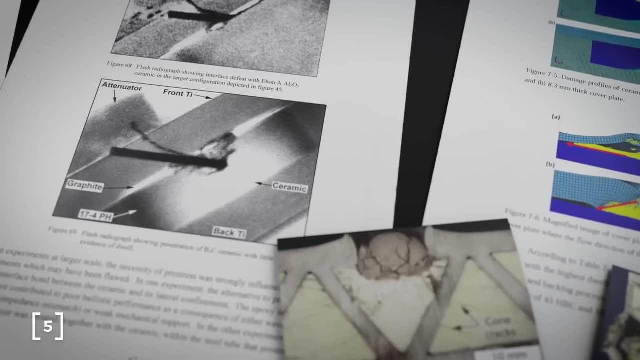 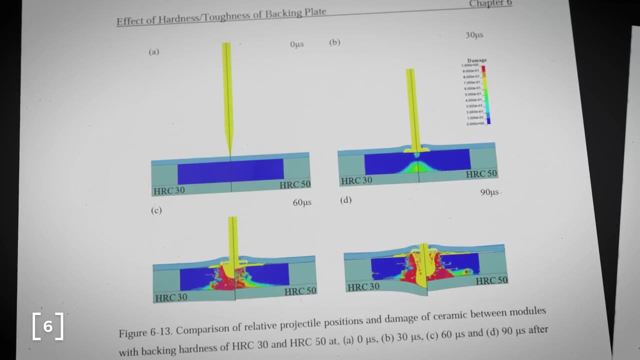 ceramic, that pulverises it and increases its volume. This creates what is essentially an abrasive maze of extremely hard and sharp particles the penetrator has to push through gradually grinding it away. Computer simulations of this effect show that the harder the material, the better. 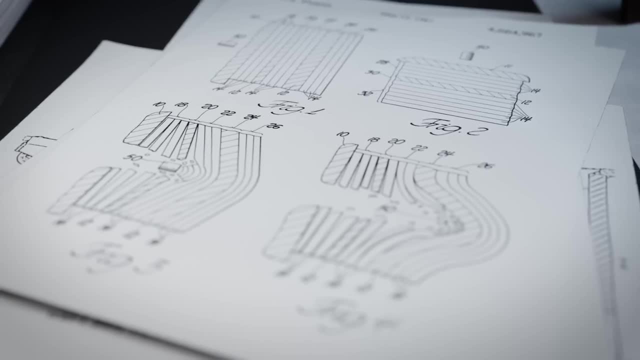 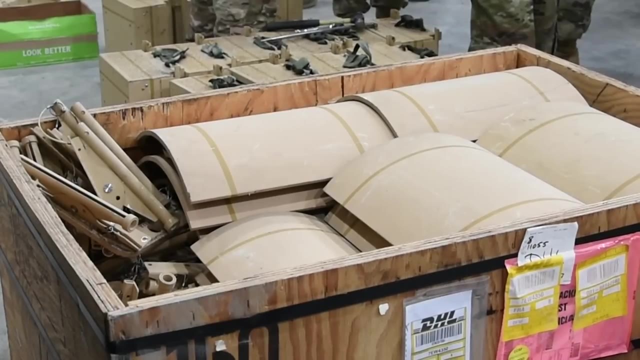 This is the magic of ceramic composite armour. This is the magic of ceramic composite armour. On top of these metal and ceramic layers, there is typically a very dense inner liner called a spall lining. Projectiles don't necessarily need to penetrate every layer of armour to be deadly. If they hit with enough force, the kinetic energy can simply transfer through the material as a wave and cause material on the inside of the tank to splinter and turn into deadly shrapnel inside the crew compartment. This is called spall. Some munitions are specifically designed to cause this. 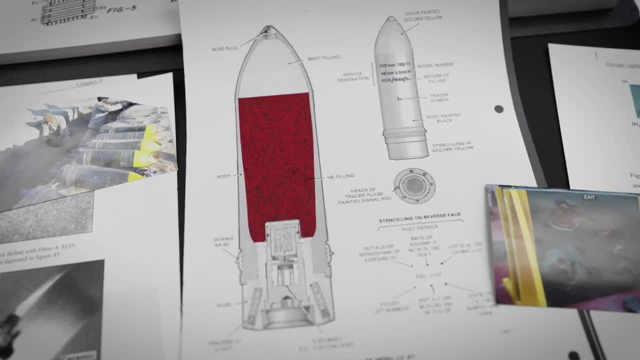 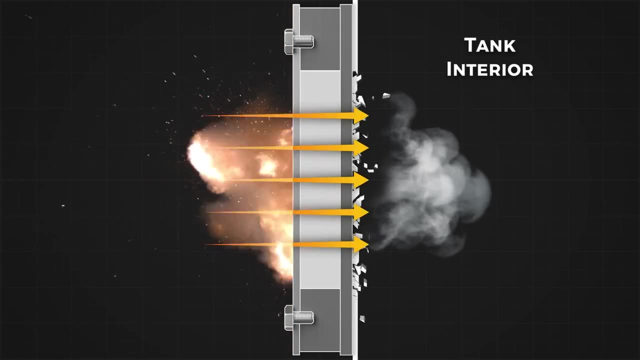 High explosive stress Squash heads are made from soft plastic explosives that spread out over the armour's surface. With the increased surface area and direct contact with the armour, the explosion transfers a great deal of energy through the material and blows out the armour's backing. 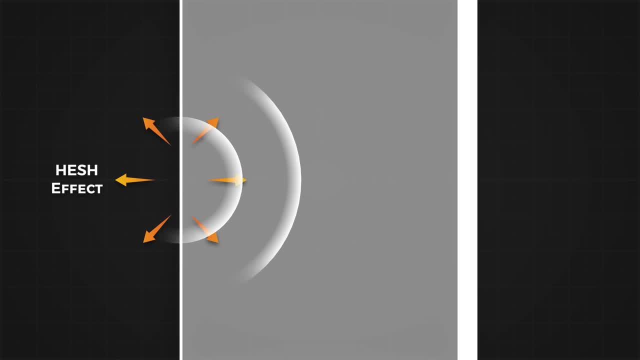 This works by sending a compressive shockwave through the material and reflects and rebounds inside the material, creating regions of intense stress that fractures the armour. The Spall Liner is a ductile and dense material that limits spalling. The Spall Liner is a ductile and dense material that limits spalling. 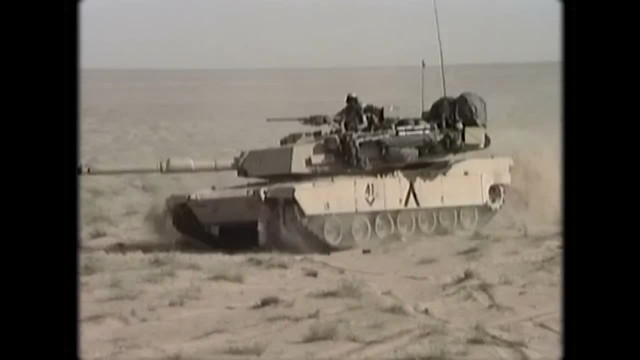 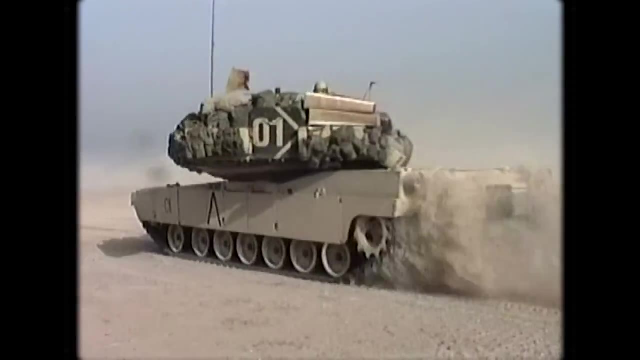 In the early M1's this layer was typically composed of lead, but beginning in 1988, certain M1A1's began to be upgraded with depleted uranium spall liners, which are even denser than lead, and all new M1A2's were assembled with depleted uranium liners. 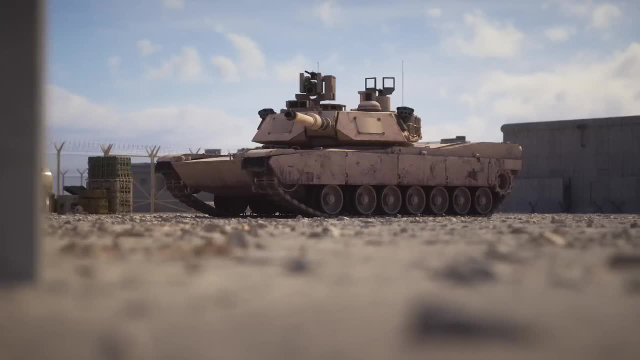 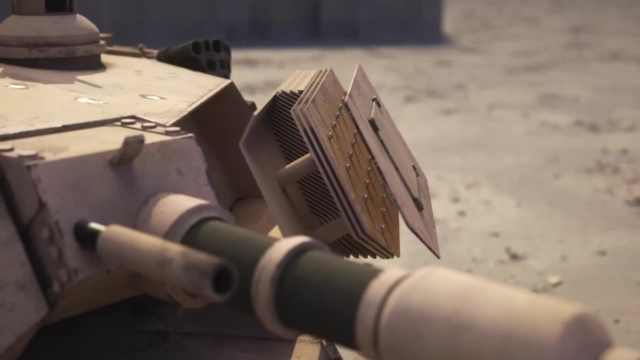 However, modern composite armour makes it difficult for this shockwave to transmit through the material, and a spaced layer with an air gap can defeat this squash head munition completely. Reactive armour tiles can be added to the outside of the M1 too. 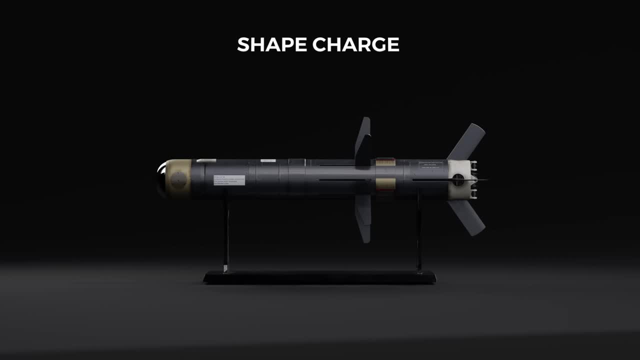 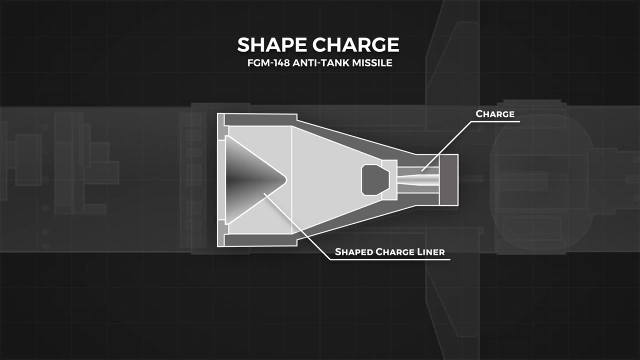 Reactive armour is particularly effective at dealing with shaped charges. Shaped charges consist of a charge shaped with a hollow indentation lined with a ductile metal liner. When the charge is detonated, a pressure wave forms behind the metal liner, deforming it. 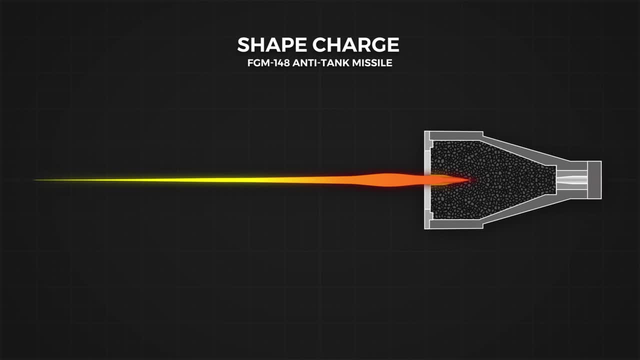 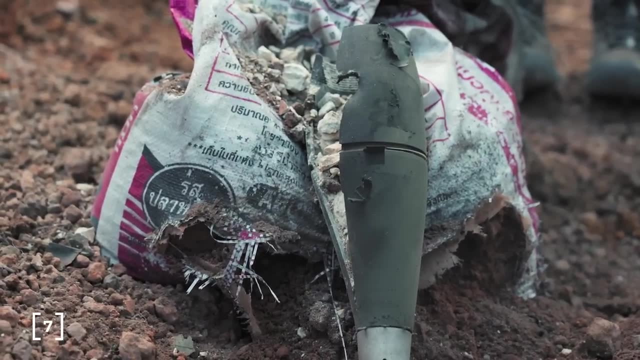 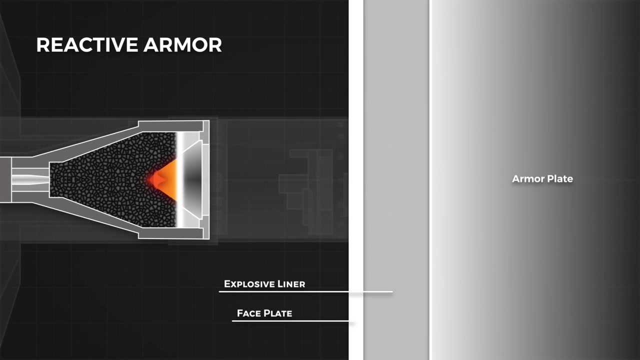 and accelerating the metal into a lance like stream of particles. The shaped charge effectively creates a hypersonic projectile at point blank range. it's highly effective at cutting through armour. Reactive armour works by placing an explosive charge between two metal plates. When a jet from a shaped charge strikes the upper plate, it detonates the inner explosive. 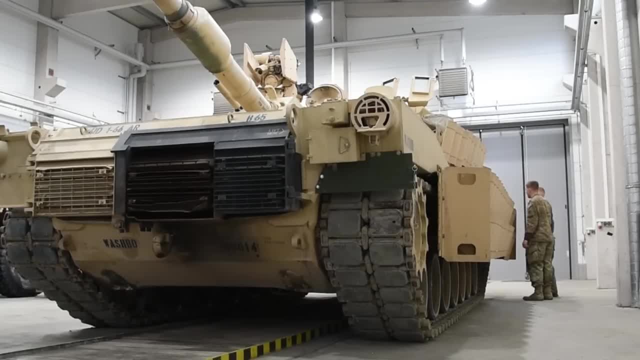 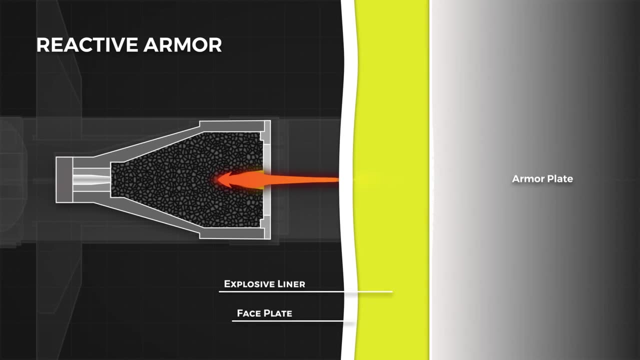 You may think this could damage the tank, but the tank's lower armour is more than capable of dealing with the relatively blunt pressure formed by the reactive armour detonation. The outer plate then flies outwards to disrupt the incoming jet while the shockwave formed. 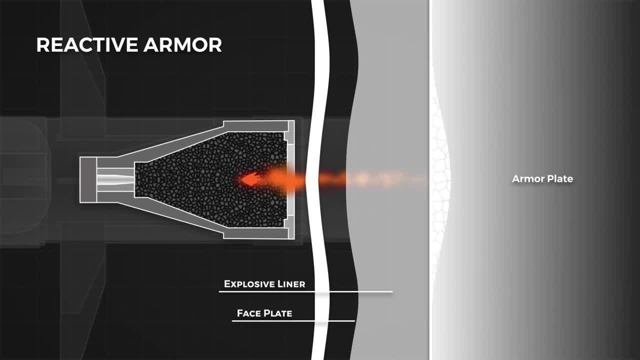 by the detonation also breaks up the stream. Reactive armour works by placing an explosive charge between two metal plates, wakes up the stream of metal approaching the tank. Of course the best defence is to not be hit at all and the M1 can create a smoke screen. 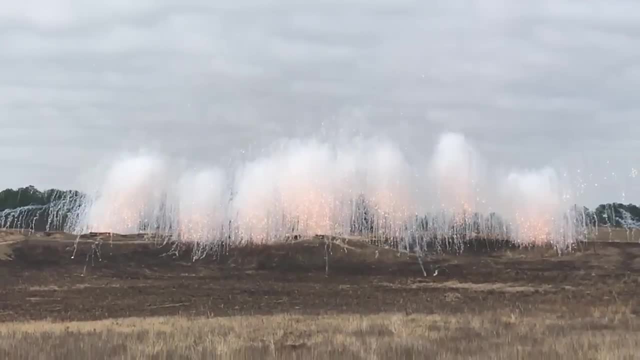 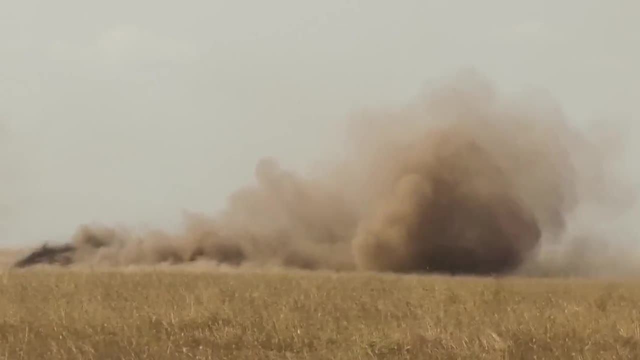 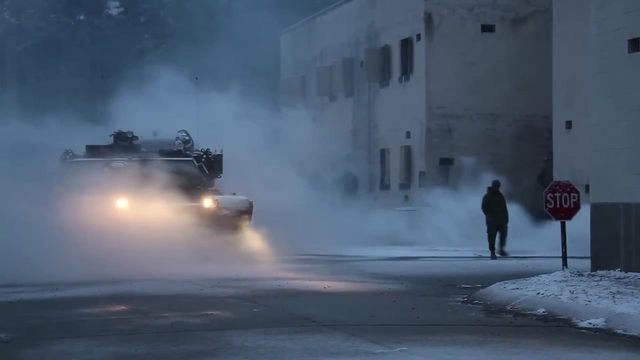 for itself when needed. The M1 has two systems for generating smoke to conceal itself in an engagement. The first involves simply spraying fuel into the engine exhaust, which vaporises the fuel and creates a large opaque cloud behind the tank. However, it's extremely important that the driver remembers which fuel the tank is running. 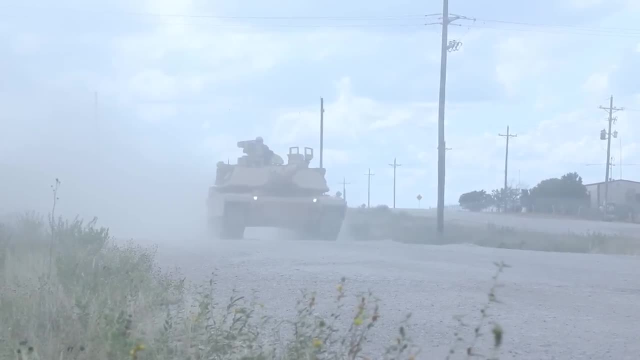 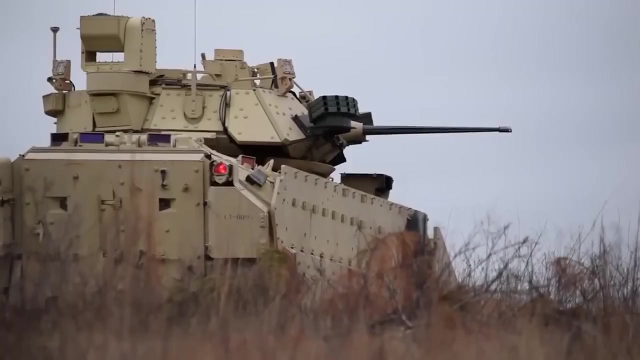 on. This works for diesel fuel, but if gasoline or kerosene is used, it won't conceal the M1, it will set it on fire. The second system uses grenade launchers mounted on the outside of the turret. There are two versions. the M1 uses 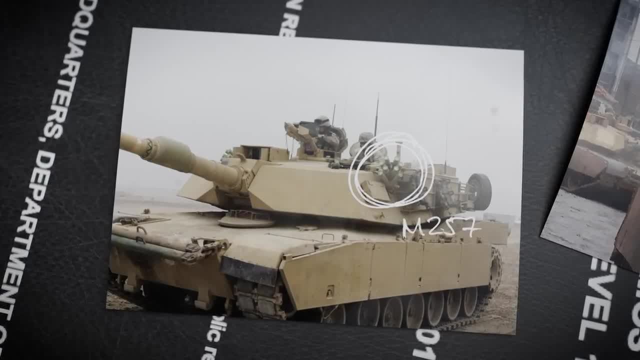 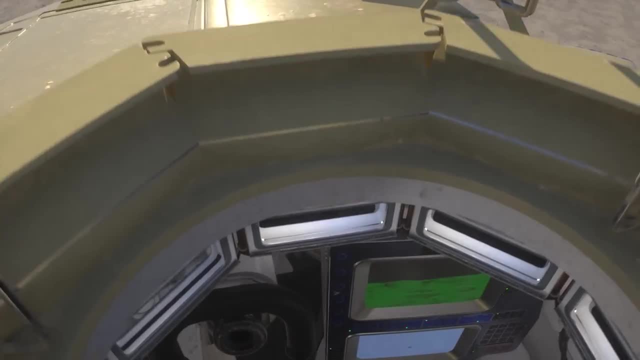 The 8 canister M257, typically used with the US Marine Corps M1's, and the more widely used 6 can M250.. These launchers are controlled from the tank commander's seat. here, Pressing one button launches 6 grenades. 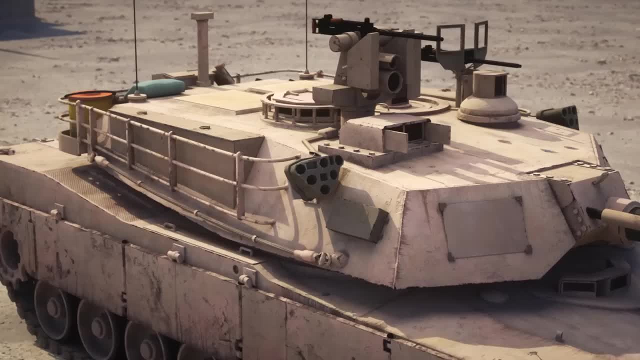 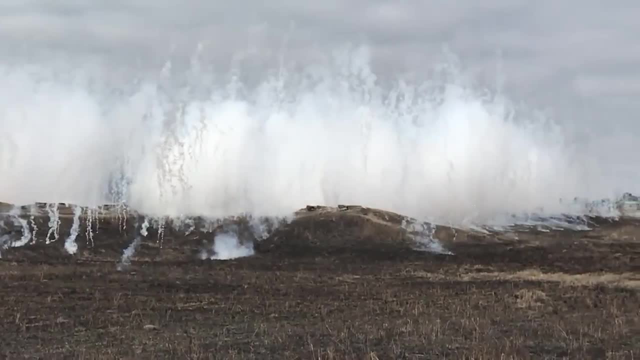 3 from the left and 3 from the right. Pressing both buttons launches all 12 of the grenades, launching them about 30 metres from the tank and providing a shrouding curtain of smoke to hide its movements. The engineers of the M1 Abrams did everything in their power to make the M1 as survivable. 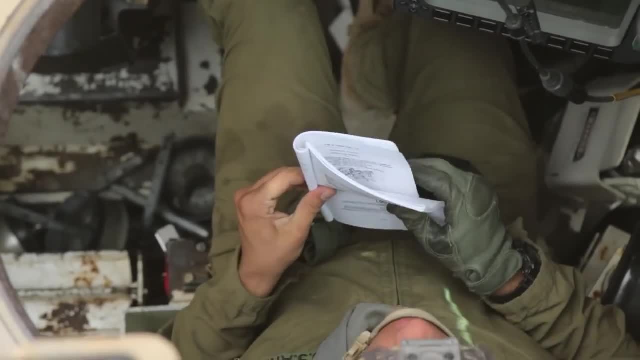 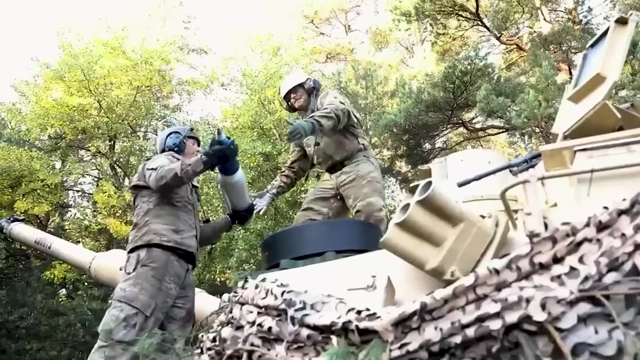 as possible. protecting the crew inside And the highly trained crew are the most important part of this machine. The M1 Abrams does not have an automatic loader. like many modern tanks, It has a dedicated crewman. The M1 Abrams is an automatic loader. 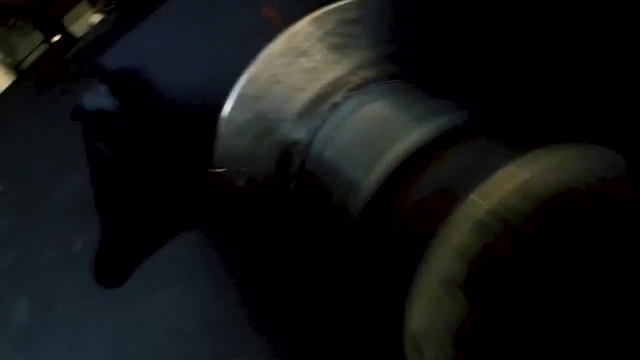 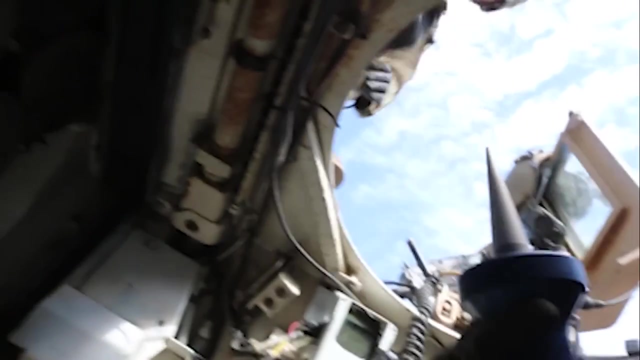 The crew member, the loader, to load rounds into the breach. Autoloaders are a feature of modern Russian tanks. However, the USA have shunned them in their tanks, Seen an autoloader as an unnecessarily complex mechanism that would impact the M1's reliability. 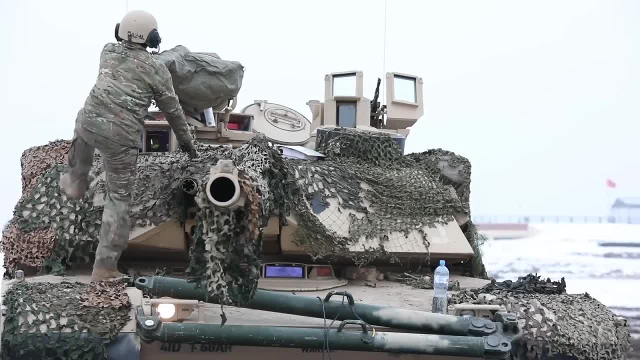 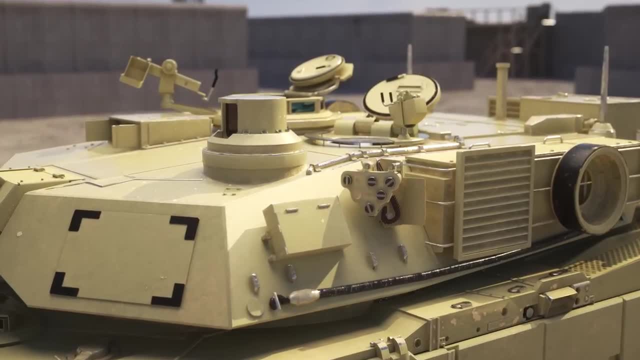 Seen a fourth crew member capable of keeping watch, maintaining the vehicle and taking over responsibilities in an emergency, as an advantage, not a disadvantage. The loader enters the tank through the turret hatch, sitting to the left of the main gun, with access to the ammunition box behind them. 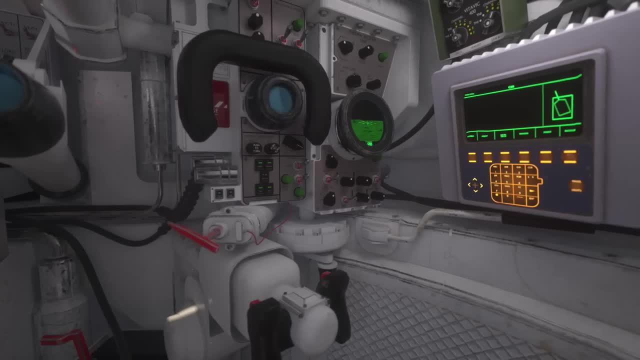 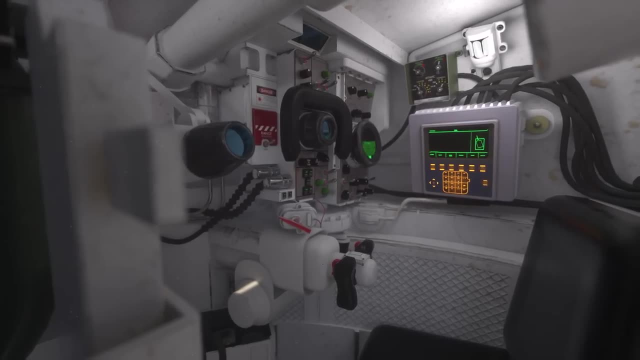 The gunner to their right, is in charge of aiming at targets using these day and thermal night vision sights, along with a laser range finder, to input target distances into the ballistic computer. When instructed by the tank commander sitting behind the gunner, the loader will press a. 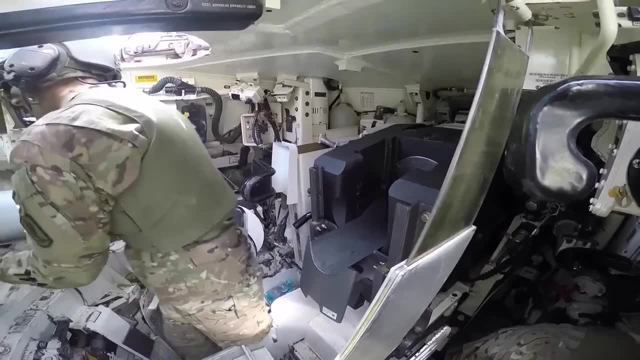 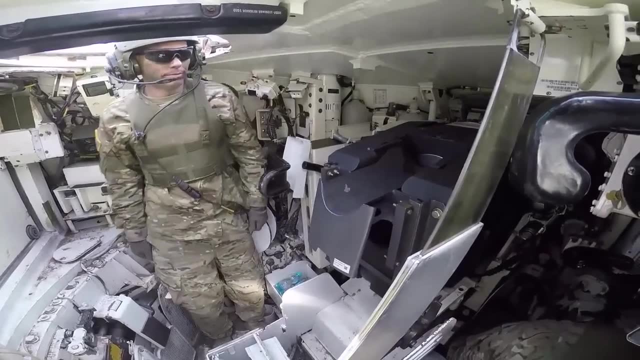 switch with their knee to open a hydraulically actuated armoured door behind them. The tank commander will specify the round needed and the loader will take it out, load it into the breech, close the breech and move the safe handle into the armed position. 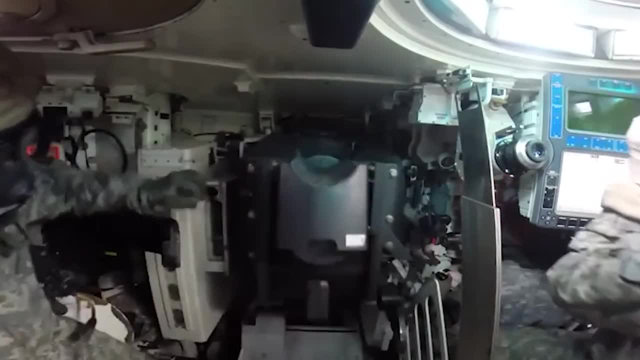 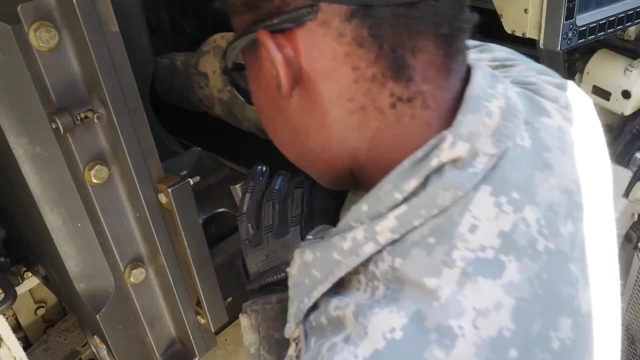 This process will be repeated until a ceasefire is called by the tank commander. The armoured ammunition access door is only open when loading, and this is crucial for the survivability of the M1 Abrams. If a round penetrates the ammunition box, it can result in a lethal detonation of the 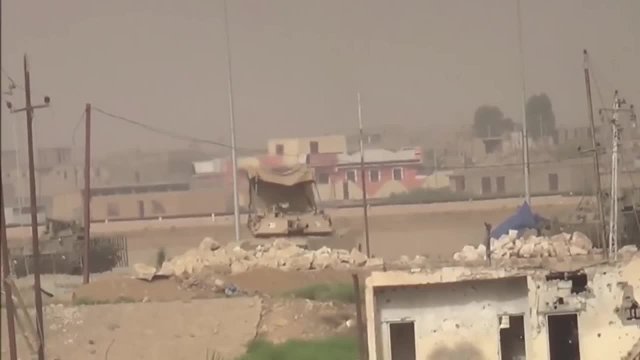 ammunition stored inside. This armoured door is capable of what's called the M1 Abrams. This armoured door is capable of what's called the M1 Abrams. This armoured door is capable of what's called the M1 Abrams. The M1 Abrams are designed to withstand this blast and panels on top of the tank called 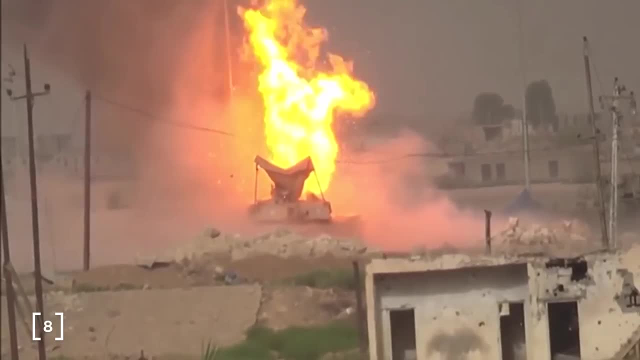 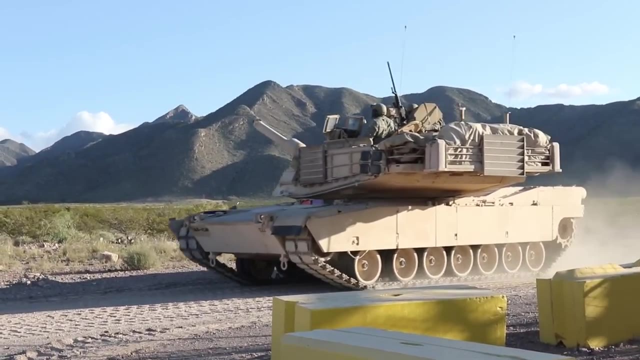 blowout panels are designed to break and allow the pressure and heat to be directed upwards and away from the crew. These rounds are fired out of the M1's 120mm cannon. Early M1's were fitted with a 105mm cannon, 105 referring to the bore diameter of the 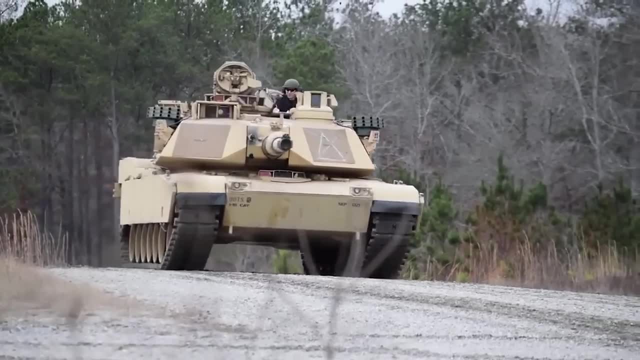 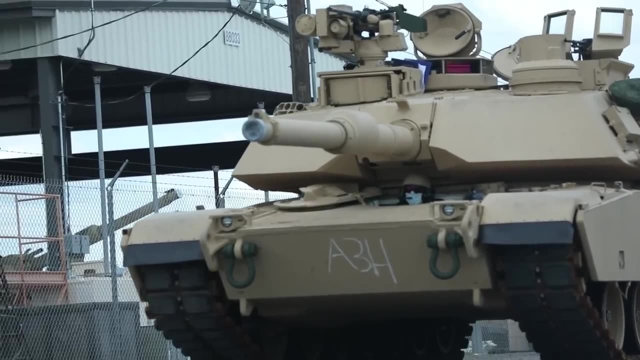 gun. This decision was made primarily to allow a sharing of ammunition and parts between the 105mm on the previous generation M16.. With the development of depleted uranium rounds, it was viewed that this gun was more than adequate to deal with any Soviet armour. 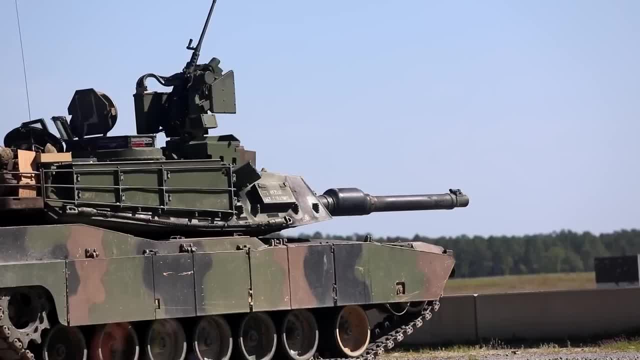 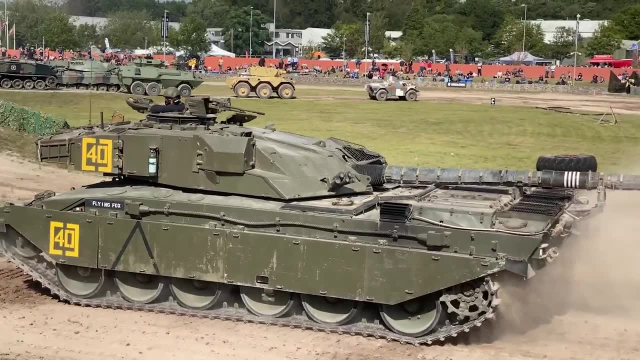 However, US allies like Germany did not want to use depleted uranium rounds due to ethical implications and were moving towards 120mm cannons, with the British Chieftain tank using the Royal Ordnance L11 and the German Leopard 2 using the Rheinmetall RH120. 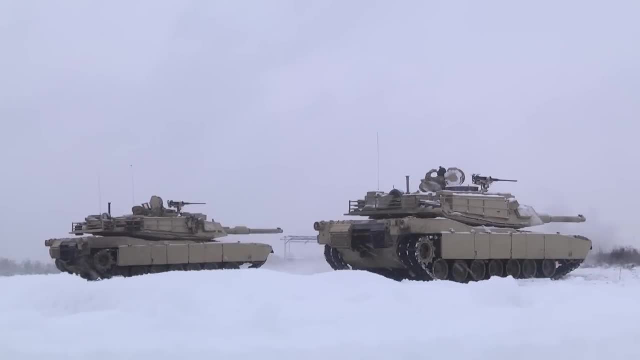 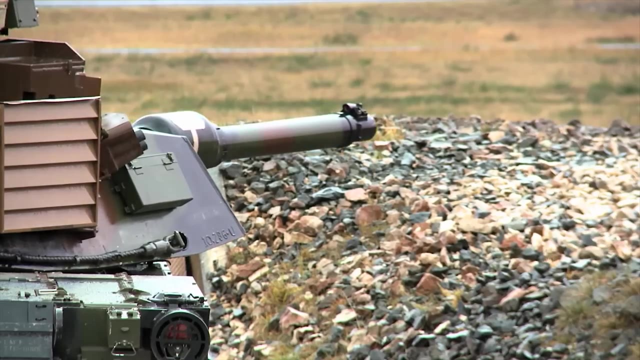 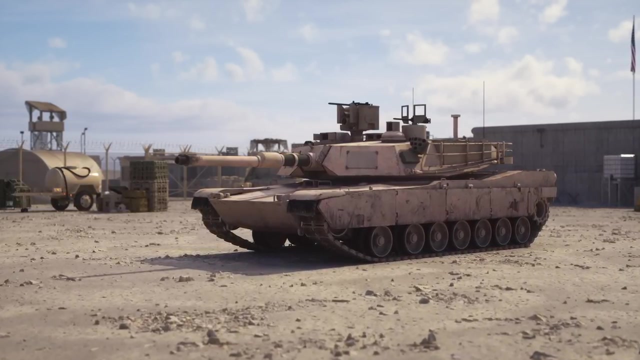 This posed a problem for NATO's goals of standardising wherever possible to optimise logistics, With ammunition factories across NATO countries producing the same ammunition. this ensured ammunition could not only be shared but manufactured as close to the front line as possible. The 120mm guns of the M1A1 and M1A2 are in fact German Rheinmetall RH120's manufactured. 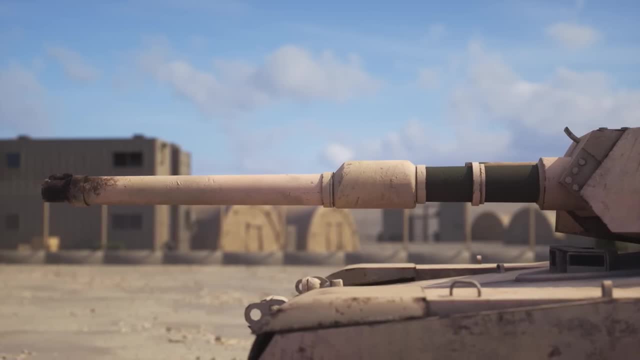 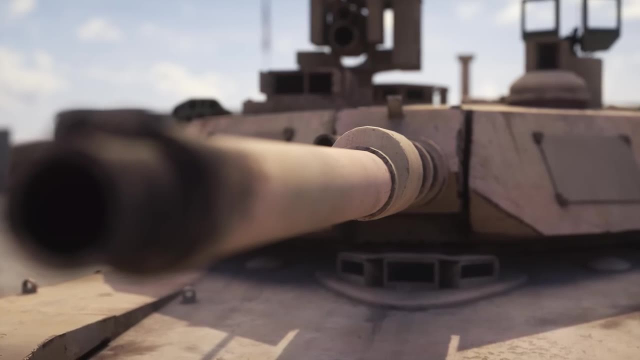 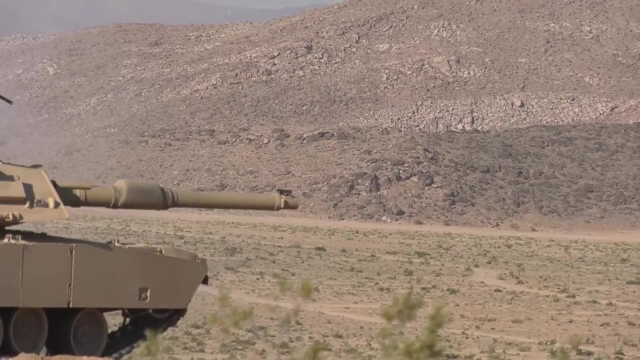 under license in the US a 5.3 metre long, 3.3 tonne smoothbore cannon. This large bulge in the middle of the cannon is designed to evacuate the barrel of propellant gases after each firing. Once the round leaves the barrel, atmospheric pressure can prevent the gases from leaving. 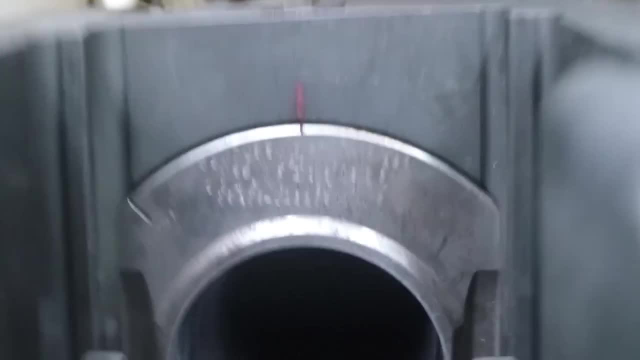 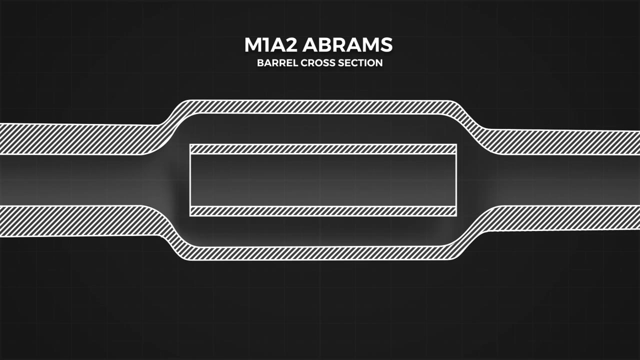 and once the breech is opened, the potentially harmful and explosive gas can enter the crew compartment. The bore evacuator is a pretty simple solution with holes that allow gases to enter the evacuator as the round passes by. This acts like a pressure reservoir. 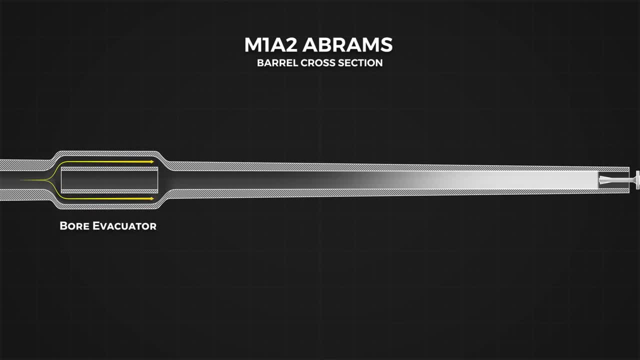 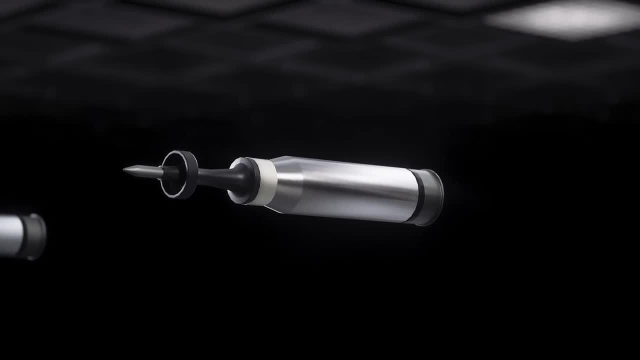 When a round leaves the barrel with this attachment, the pressure is released from the forward-facing holes at the far end of the evacuator and this pushes the remaining gases outwards. The two primary rounds used by the M1 are the M829 depleted uranium round, which is 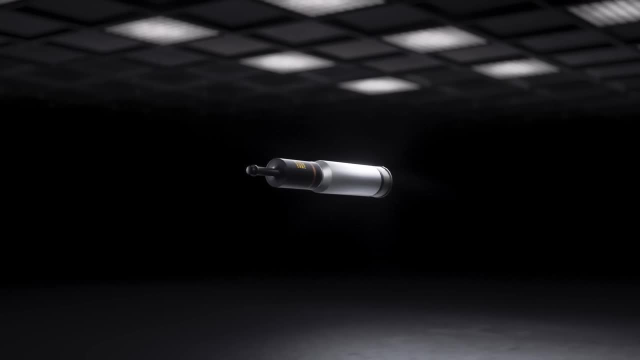 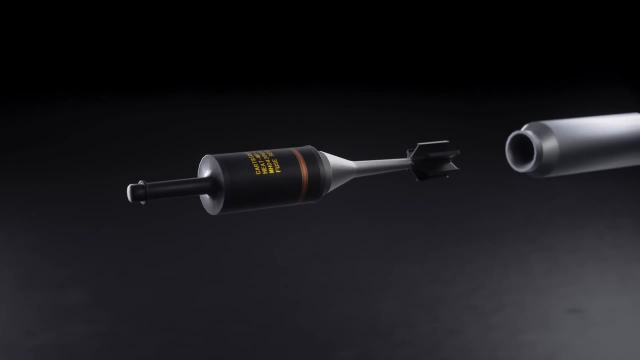 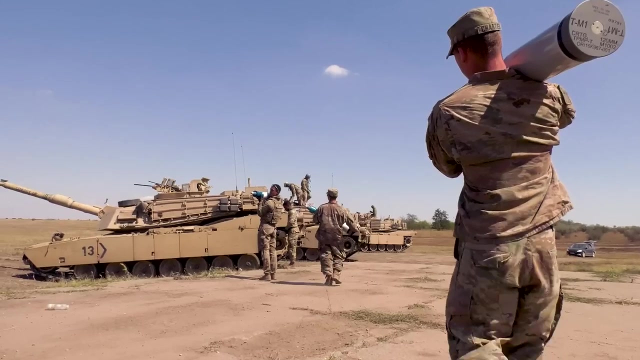 a sabot kinetic energy round and the M830A1 heat round which, despite its name, does not use heat as part of its offensive. It uses a kinetic energy shaped charge. We have been piling on weight in this vehicle. The armour, cannon, engine and ammunition makes this an extremely heavy vehicle weighing. 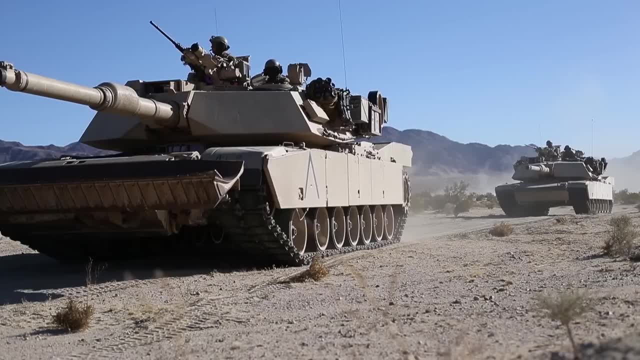 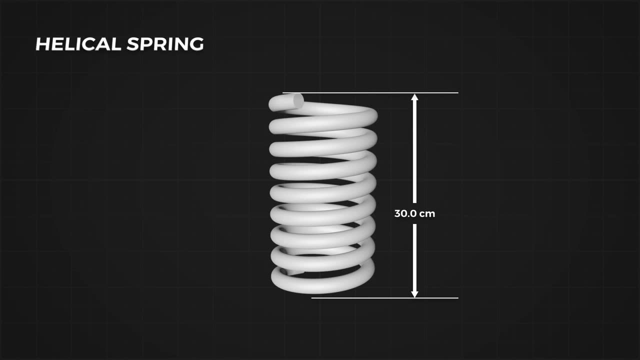 between 52 and 68 tonnes, depending on the generation and configuration. The M1 Abrams needed a track and suspension system capable of bearing that weight For a vehicle. this heavy typical helical springs have some problems. First, their maximum travel is limited. 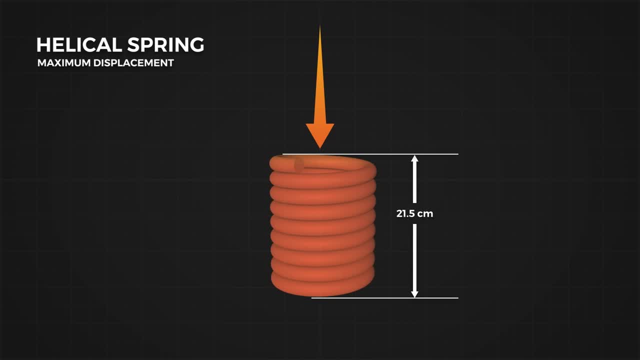 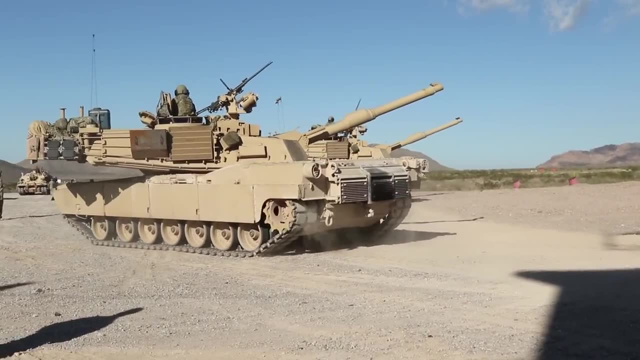 At a particular load, the layers of a helical spring will meet and no further travel is possible. This means coming out and providing an extremely uncomfortable ride for the crew. To deal with a heavier vehicle, we need to increase the spring coil diameter taking. 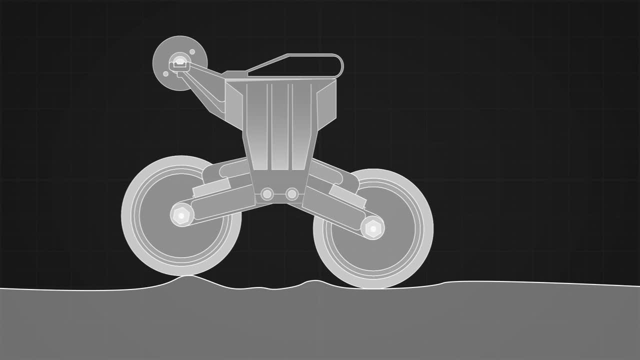 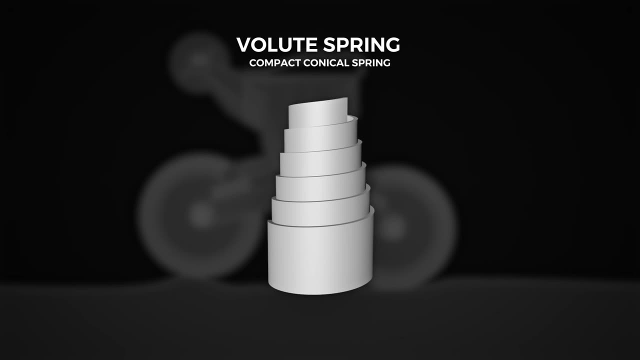 up an increasing amount of space. This was an issue for World War 2 era tanks, with the M4 Sherman opting to use a volute spring, which is a conical spring that is capable of compressing to a much smaller size as the sheets of spring steel overlap. 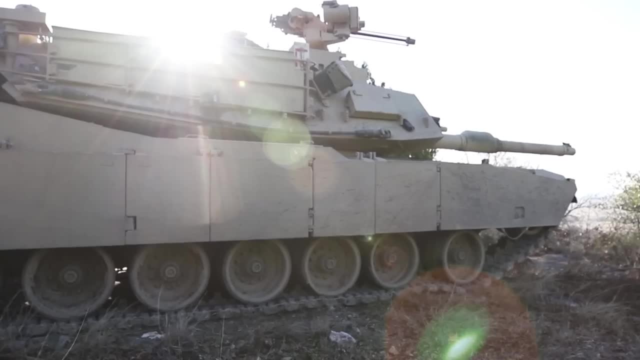 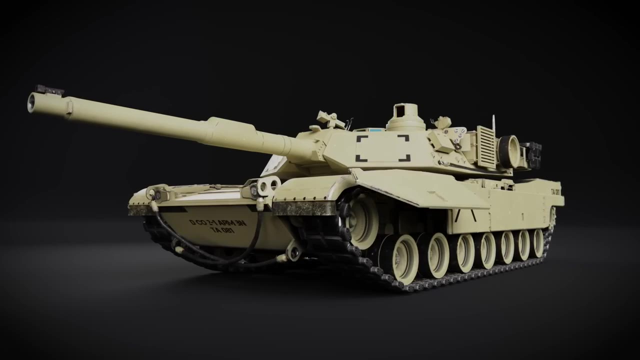 However, most modern tanks utilise the torsion spring, which take up very little space inside the tank, though they do raise the tanks height considerably. The torsion springs of the M1 are located here and because they are inside the hull, they raise the hull height by 150 millimetres. 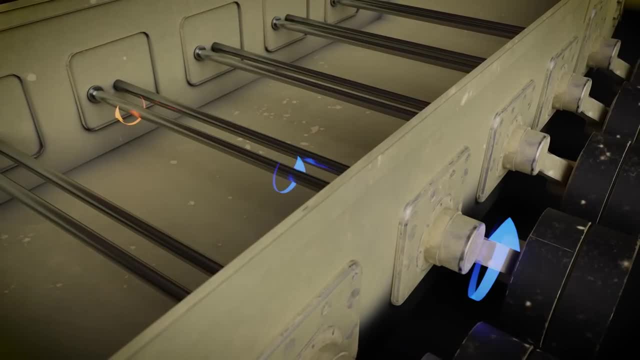 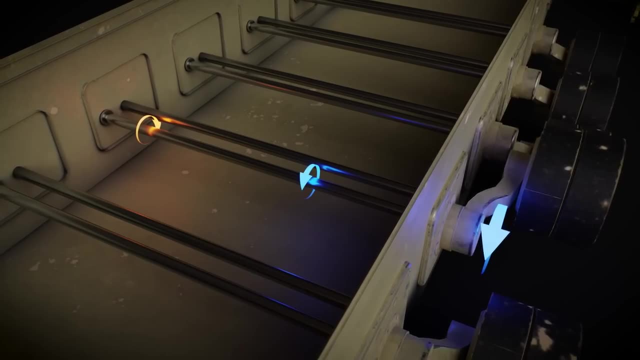 The road wheel is attached to a lever which can travel up and down. This lever arm is attached to the torsion bar so that it twists when the lever arm moves up and down. The spring force is derived from the bar's resistance to torsion. 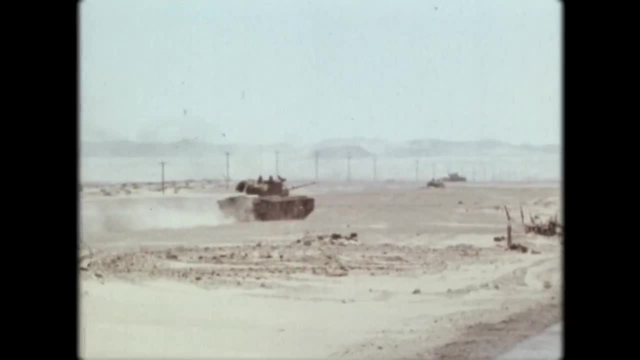 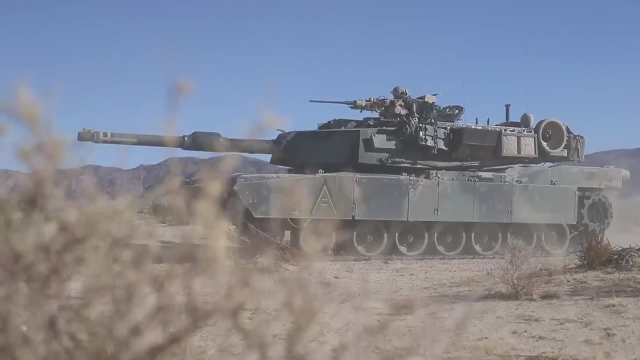 Older tanks incorporating torsion bars had limited travel. The M1's predecessor, the M1A1A, was used as a torsion spring. The predecessor, the M60, had a wheel travel of just 20 centimetres. During the development of the M1, the two tanks were pitted against each other. 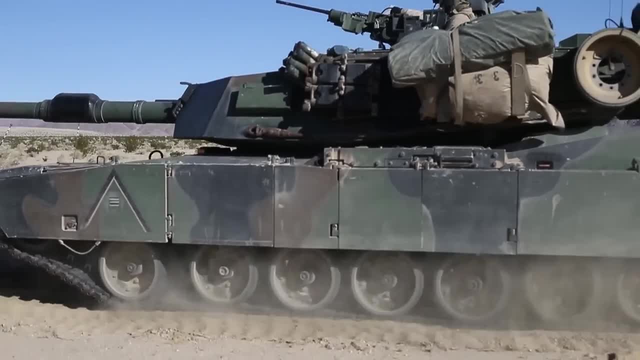 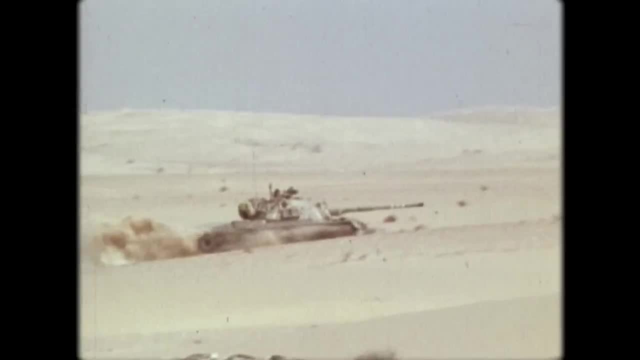 With the M1 benefiting from 20 years of material science progress. its max travel was nearly double that of the M60, at 38 centimetres, When tested on a track with a series of 30 centimetre bumps, at 32 kilometres per hour. 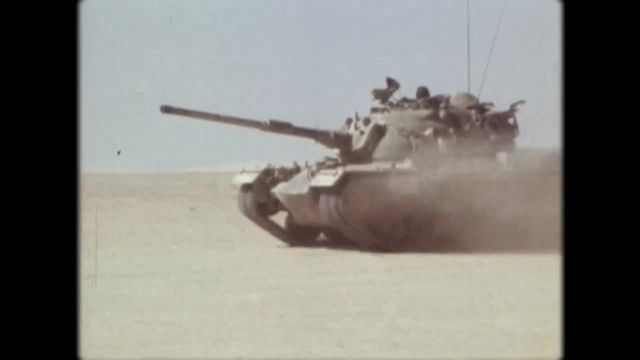 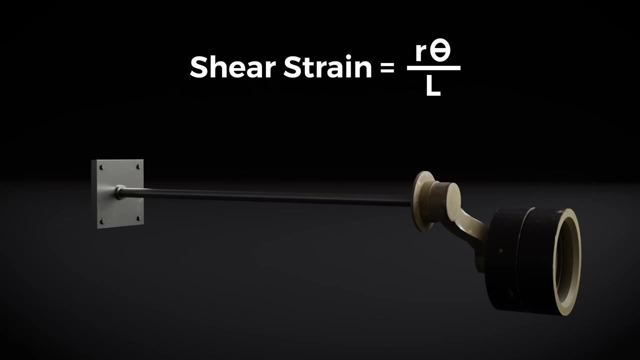 the M60 managed to break its front wheels, lost control and broke the driver's arm. The torsion spring of the M1 runs through the front wheels. The torsion spring of the M1 runs through the front wheels. The torsion spring of the M1 runs along the width of the hull, making them quite heavy. 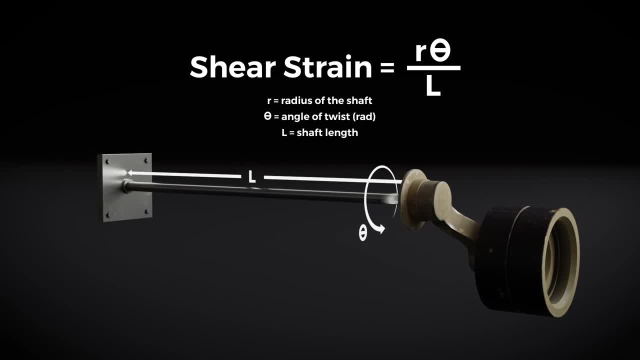 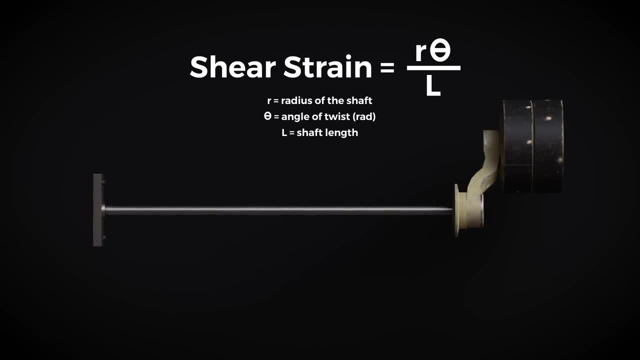 We need the torsion spring to be as long as possible, because the travel distance is a function of the torsion bar's length. Longer torsion bars can twist more before breaking. An interesting quirk of the torsion spring system is that typical designs like the M1's 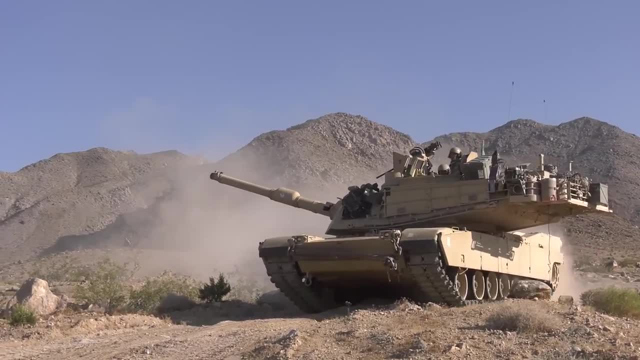 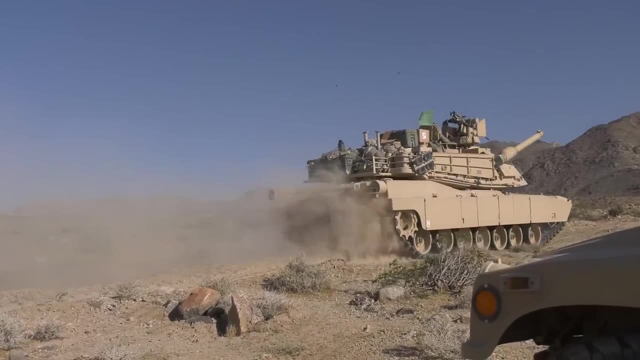 mean that the road wheels cannot be aligned. We cannot connect the lever arms of opposite road wheels to the same torsion spring, as they would frequently travel together, creating no torsion. The far end of the bar needs to be rigidly mounted to the body of the tank in order to 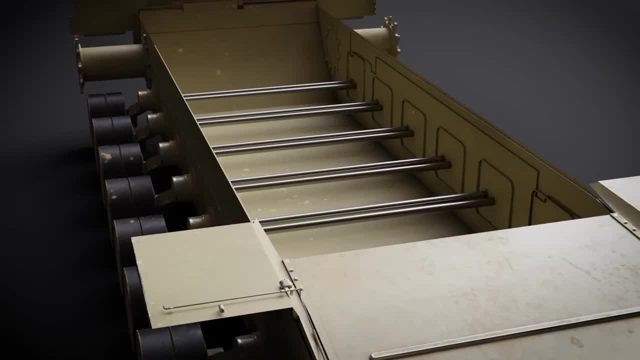 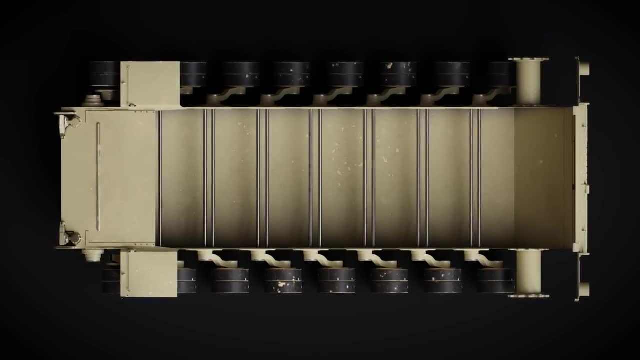 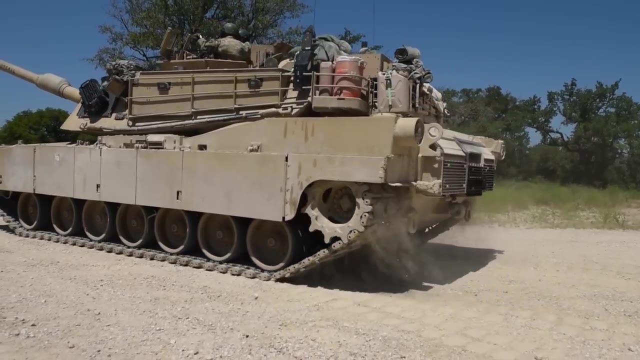 develop a spring force, So two torsion bars need to be mounted alongside each other, creating an offset in distance between the two sides of the tracks. The two sides of the M1 are not symmetrical. This comes with some drawbacks. The leading road wheel will hit bumps first, meaning it will absorb more force than the 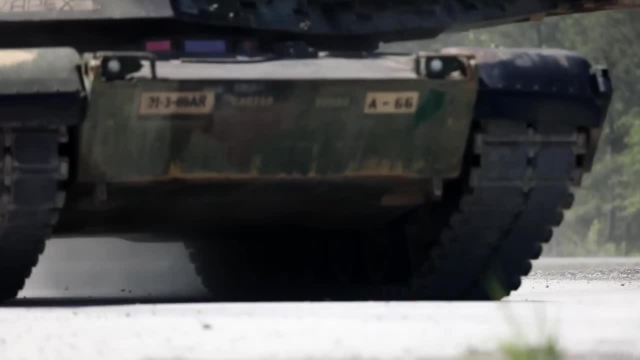 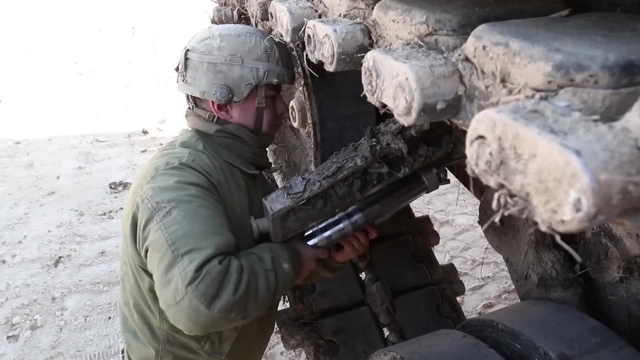 trailing road wheel, Increasing the wear on the leading torsion spring, resulting in more frequent replacements. Torsion bars are very easy to swap out when they aren't broken, but if bent or shattered, or if the body of the tank is bent, it can be difficult to pull the long torsion springs. 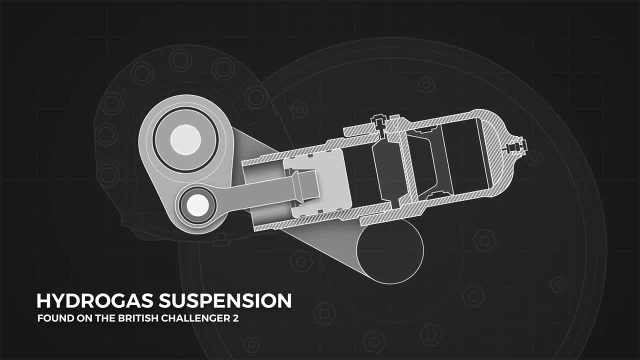 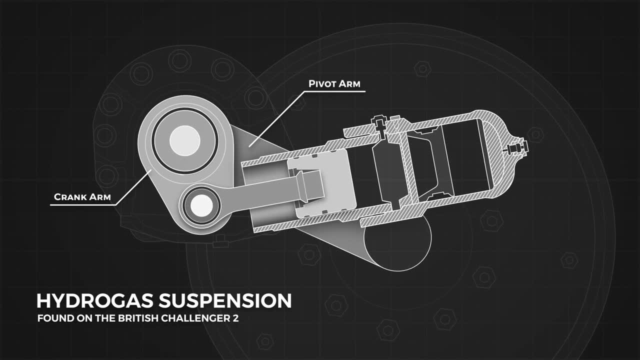 out. Modern tanks are increasingly moving towards hydro gas suspensions which look like this: The road wheel has an attached axle pivot arm which in turn turns a crank and a con rod piston. This piston connects to a hydro gas suspension. This piston is also connected to a con rod piston. 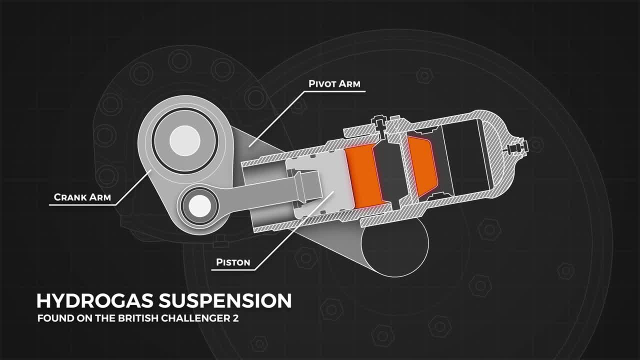 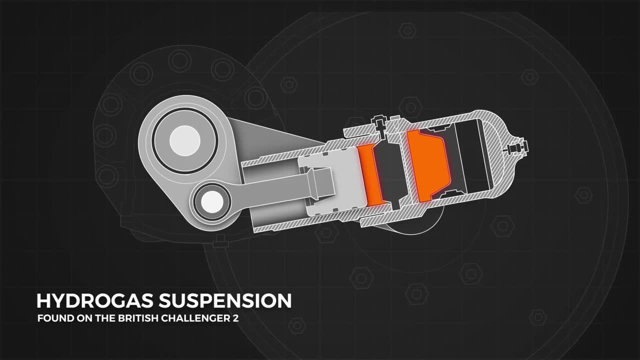 This piston connects to a hydro gas suspension. This piston is also connected to a con rod piston. The first chamber is filled with fluid, typically oil. The oil is relatively incompressible, and so this provides marginal spring force, But this chamber has a Damper Valve that serves to restrict the transfer of fluid between. 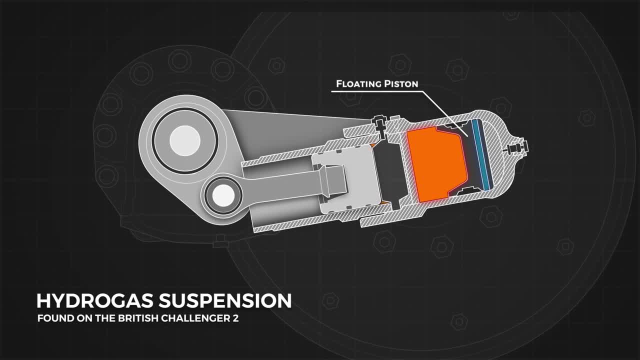 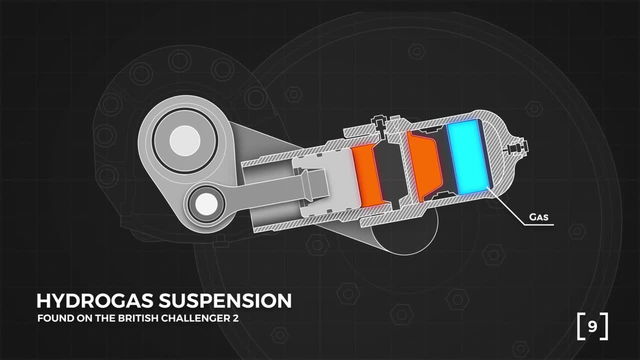 this chamber and the next, which contains a floating piston with a compressed nitrogen gas on the other side. This provides the spring force to ensure the road wheels stay in contact with the ground, but also dampens out vibrations. This system is much smaller, lighter and has a small first install ahead. 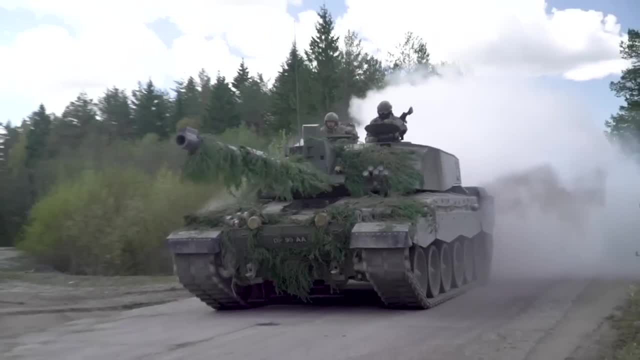 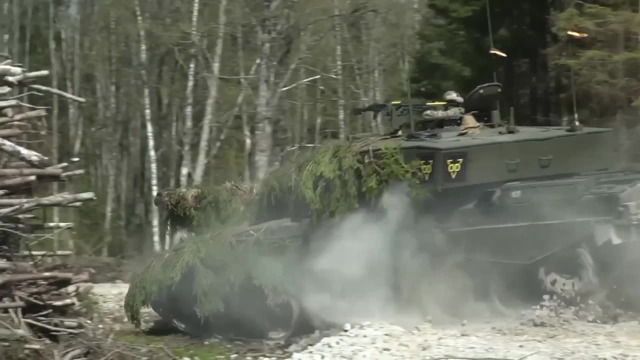 smaller, lighter and easier to service than torsion bars, while lowering the height of the tank, lowering its profile and making it harder to hit. Not only that, but each individual suspension can be remotely adjusted by changing the gas pressure inside the cylinder. 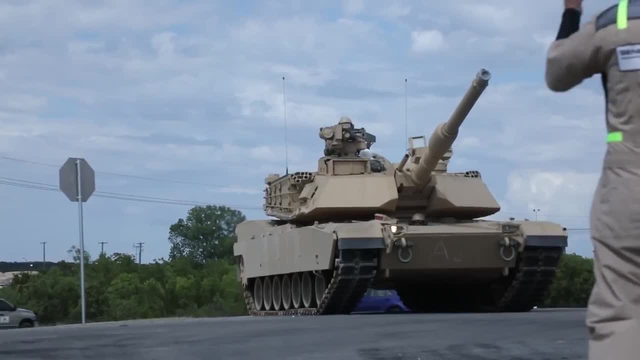 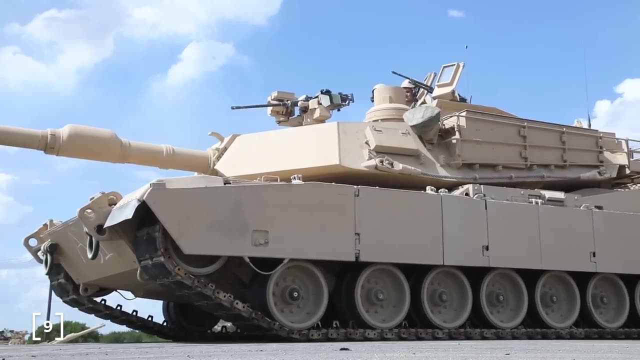 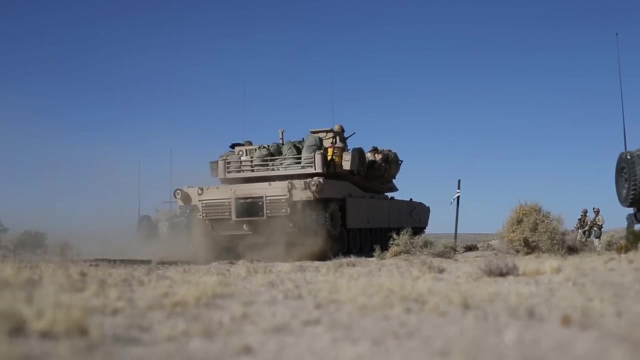 allowing the tank to take a crouch position if needed. Hydrogas suspensions were considered for the M1 during development, but it was a relatively new technology at the time and so the torsion spring was chosen. The M1 Abrams has had incremental improvements added over the past four decades, with three 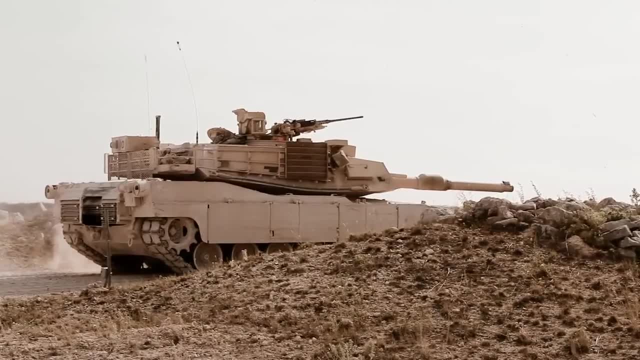 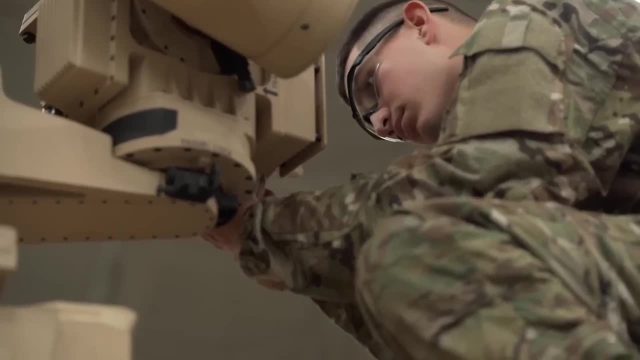 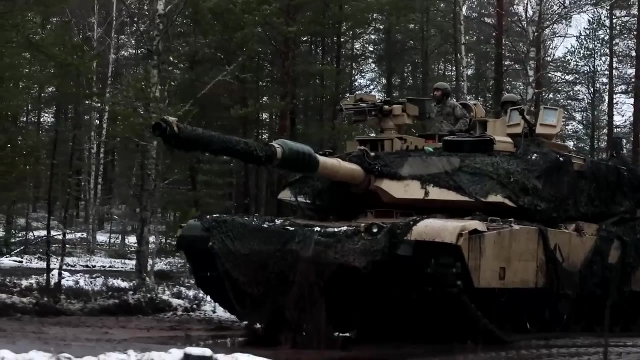 primary variants: the M1, M1A1 and the M1A2, with even more specialised iterations in between, With updated sensors and controls to bring the tank into the 21st century, like the CROWS 2 on the M1A2. SEP. SEP standing for Systems Enhancement Package, which added additional. 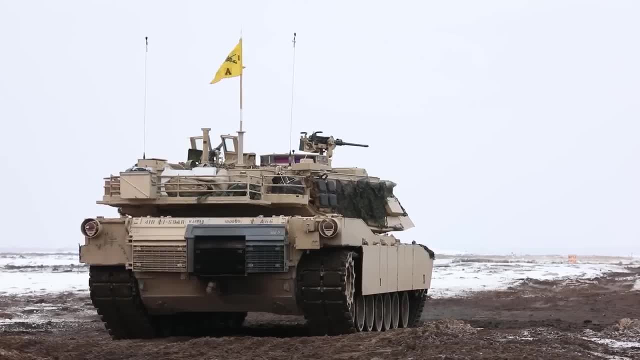 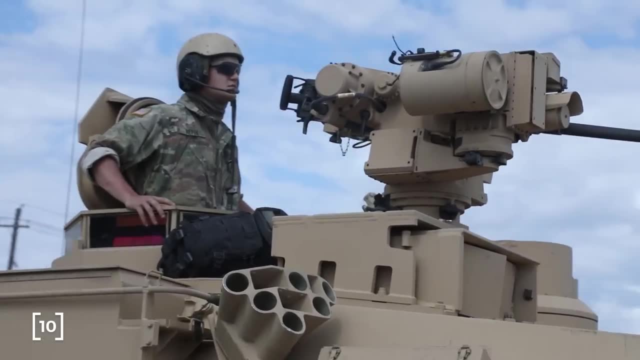 thermal sights for the tank commander, an auxiliary power unit to run its electronics without running the fuel hungry engine, and the CROWS 2 controller, a remote control site that allows the tank commander to operate the gun from the safety of the turret. 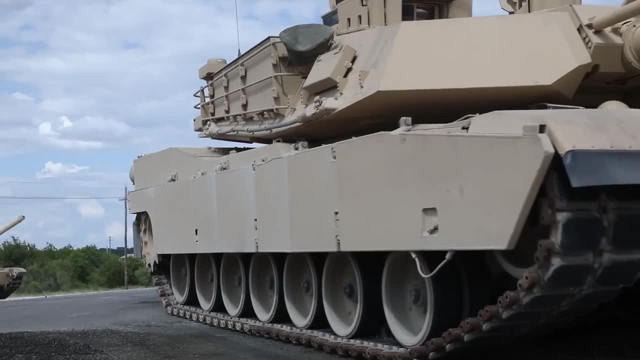 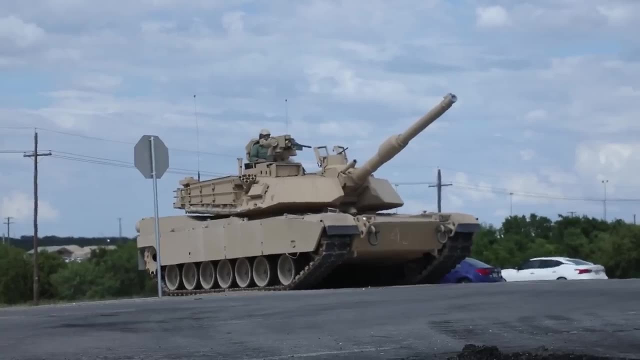 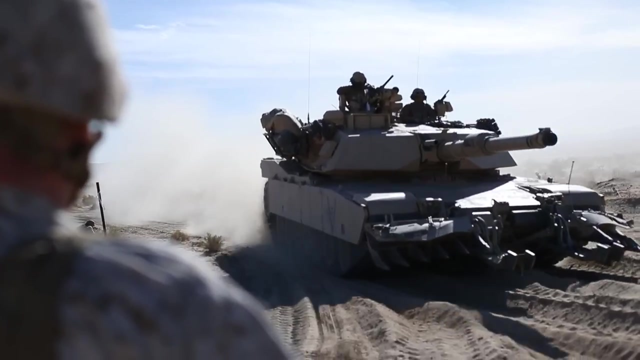 We are currently on the M1A2 SEP V4 variant and the army is considering the future of the M1 program, whether that's the M1A2, SEP V5, or a completely new platform. But make no mistake, despite the M1 being one of the longest serving tanks in a modern military, 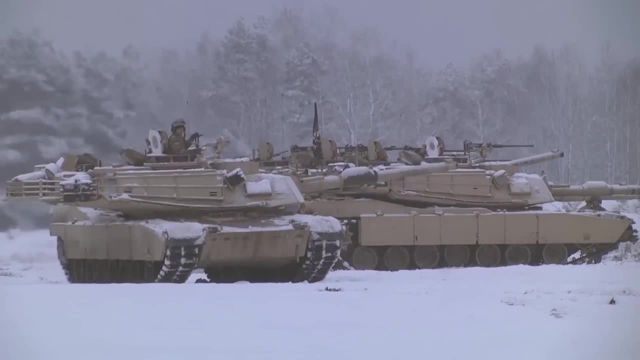 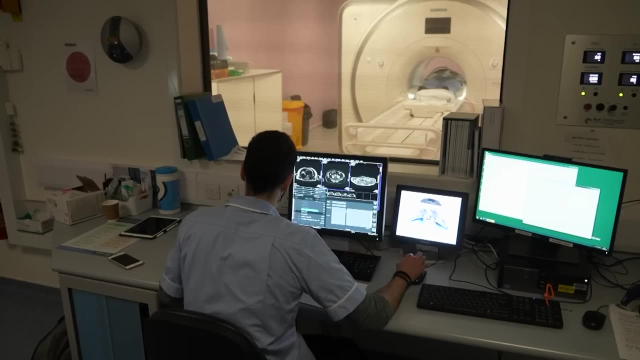 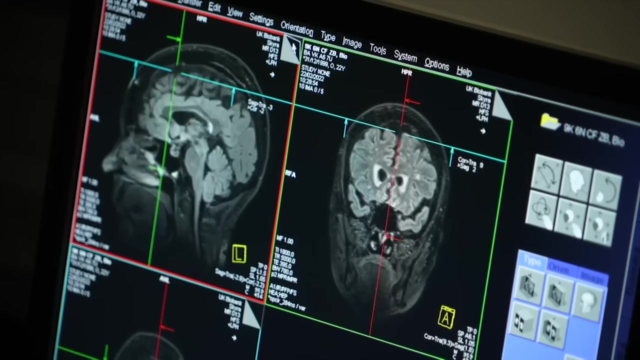 over four decades old, It's still highly capable and will be a massive asset to the troops on the ground in Ukraine. The next episode of Real Engineering is about the incredible physics behind Magnetic Resonance Imaging. It will be out on YouTube in two weeks, but maybe you want to prepare in advance. 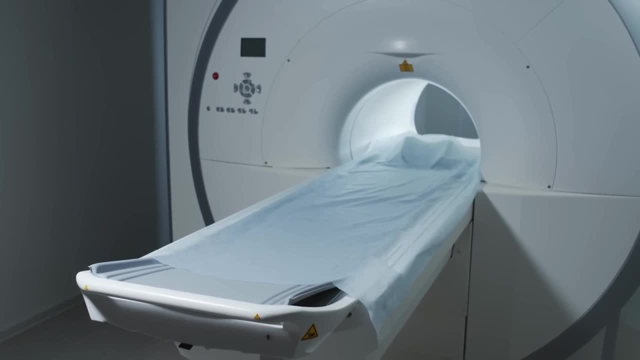 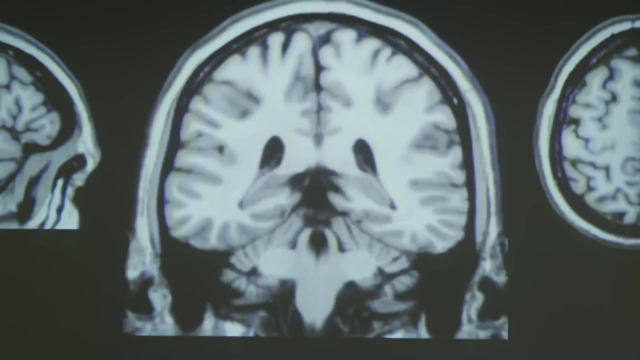 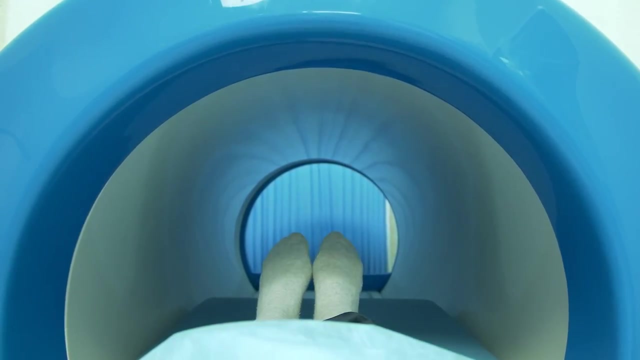 to better understand what we talk about. MRI machines use a pretty incredible property innate to our body tissues: the quantum spin of hydrogen atoms and how they interact in different tissue types. It took us a long time to write this script. Understanding quantum mechanics is hard and